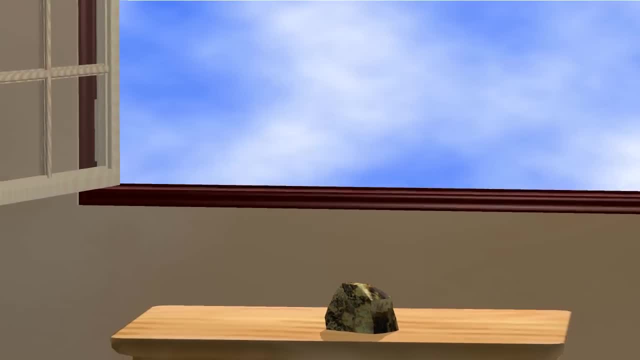 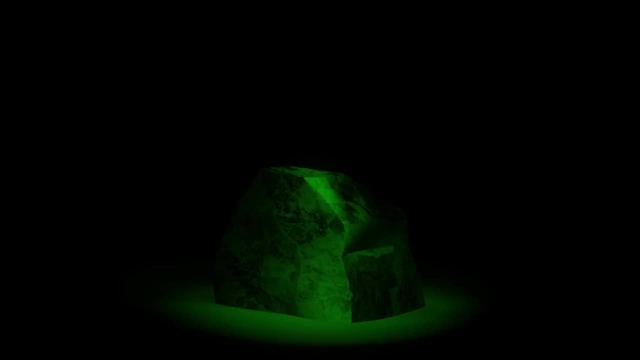 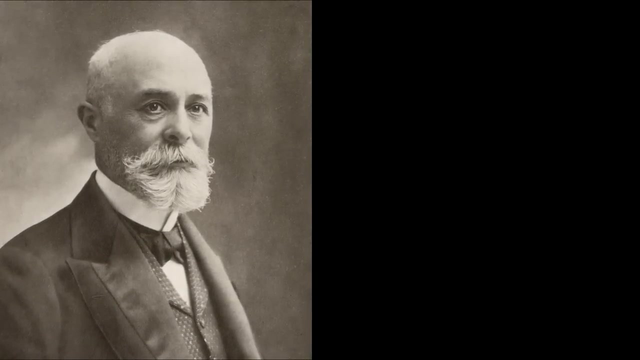 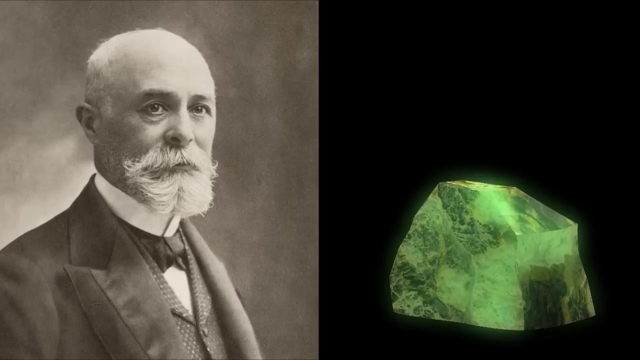 of uranium, whereby the rock mineral would give off visible light in a darkened room for minutes to hours after exposing the stone to sunlight. Professor Becquerel, working with a crystalline crust of the phosphorescent material potassium uranyl sulfate, suggested that, in addition to the familiar visible phosphorescence that 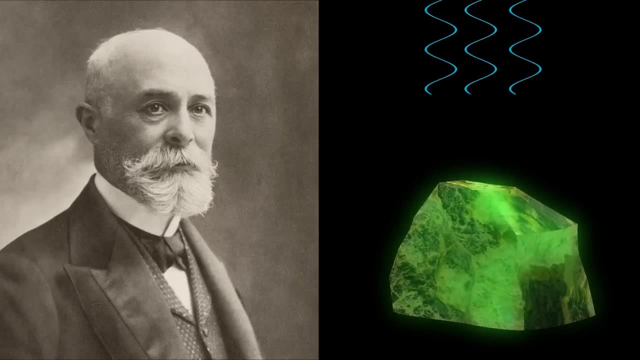 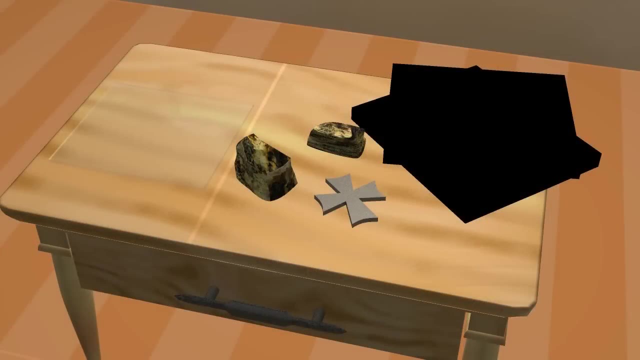 these substances could possibly emit some of the mysterious new penetrating rays described by Roentgen a few months earlier. To test his hypothesis, Becquerel wrapped a photographic plate coated with a silver bromide emulsion and two sheets of very thick black paper to be used to destroy the 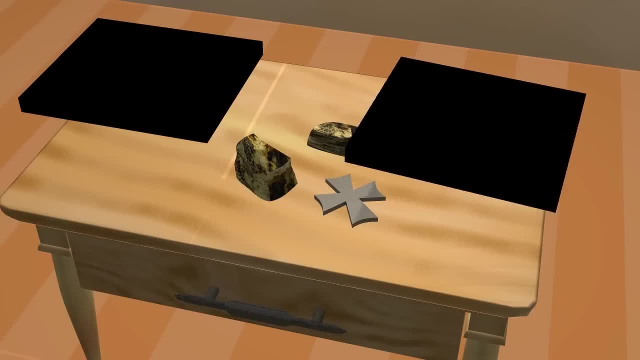 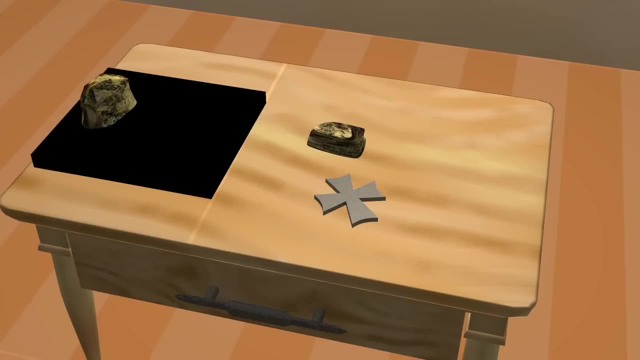 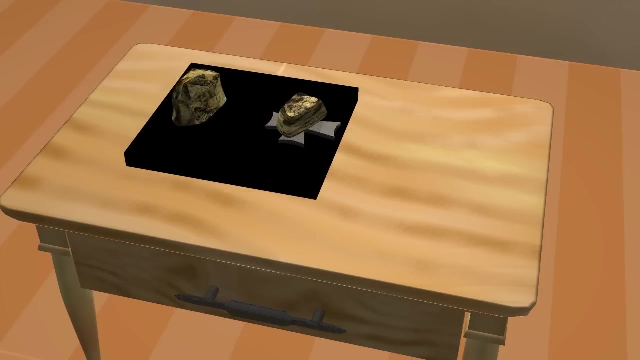 to prevent fogging from direct sunlight. He then placed slabs of the uranium salt on top of the black paper, some directly on the paper and others on a piece of money or metal screen. The entire apparatus was then placed in the Sun for several hours. 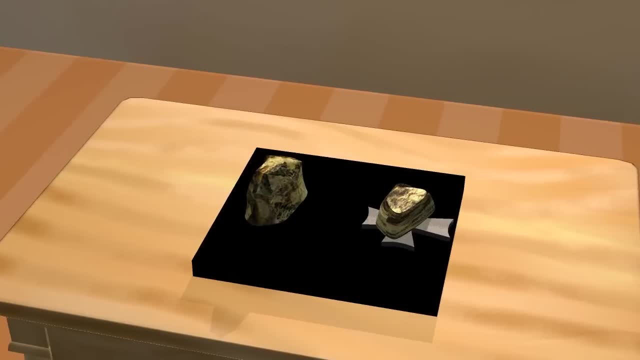 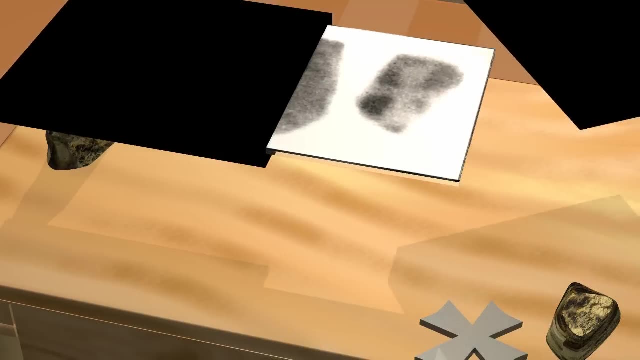 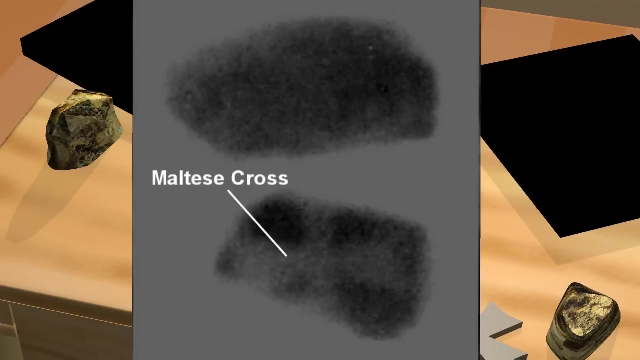 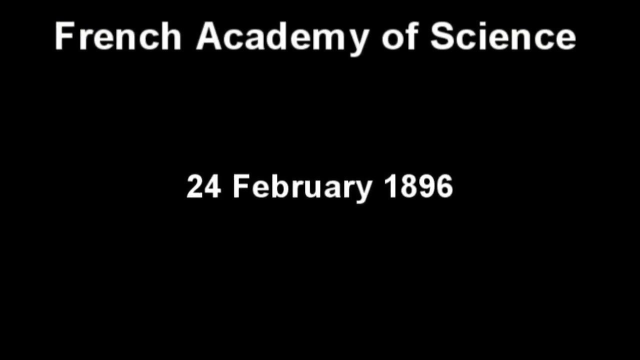 Developing the photographic plate, Becquerel identified the silhouette of the stones in black with the metallic objects, like this Maltese cross, appearing in the negative. Becquerel described his findings to the French Academy of Science on 24 February 1896, concluding that from these experiments it is evident that the 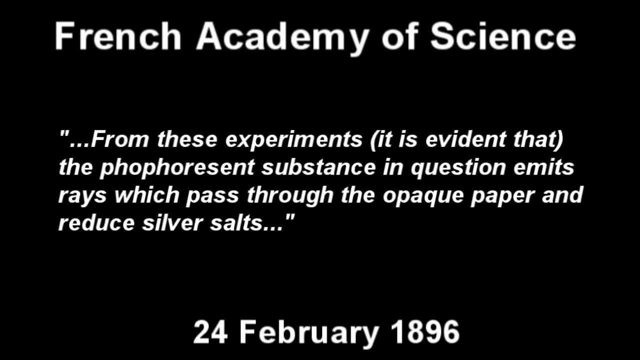 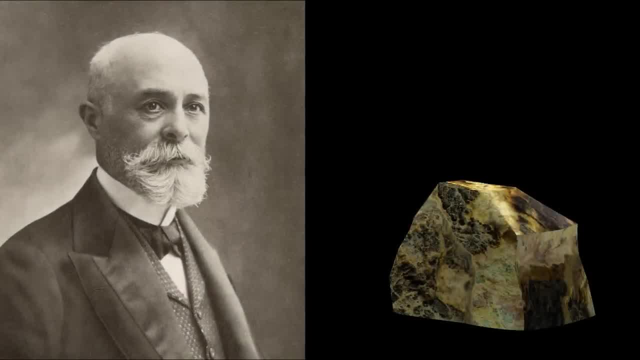 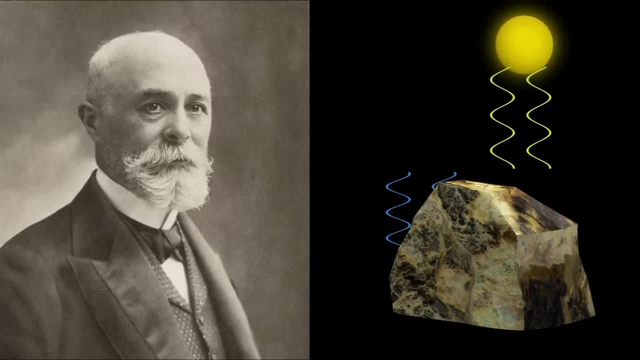 phosphorescent substance in question emits rays which pass through the opaque paper and reduce silver salts. At this point, Becquerel was certain that the observed phenomenon was the result of the uranium crystals ability to absorb energy from the Sun and re-emit that energy in the form of the identified penetrating rays. 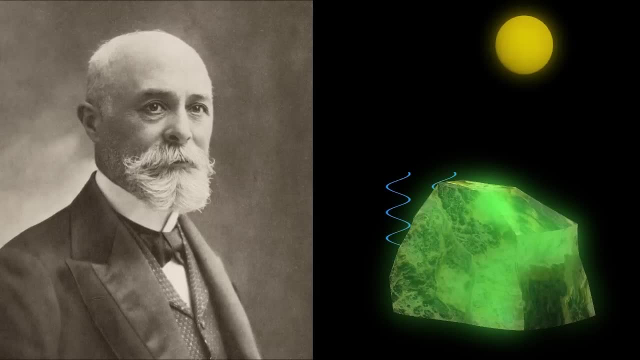 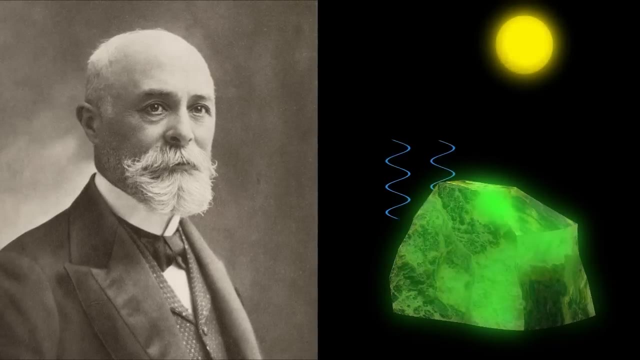 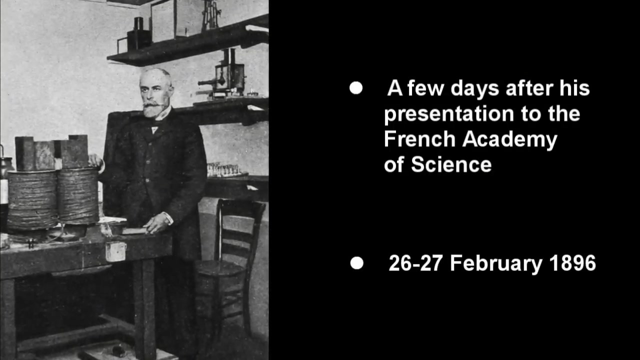 However, further investigations and a fortuitous streak of bad weather on the last few days of February 1896 caused him to abandon that hypothesis A few days after his presentation to the French Academy on the 26th and 27th of February 1896,. 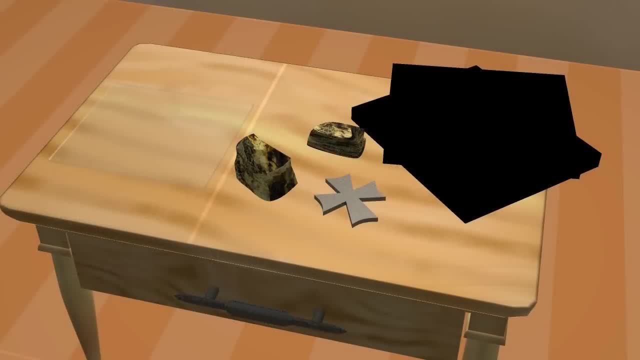 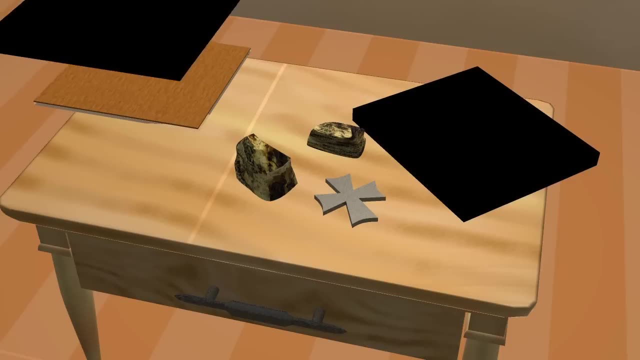 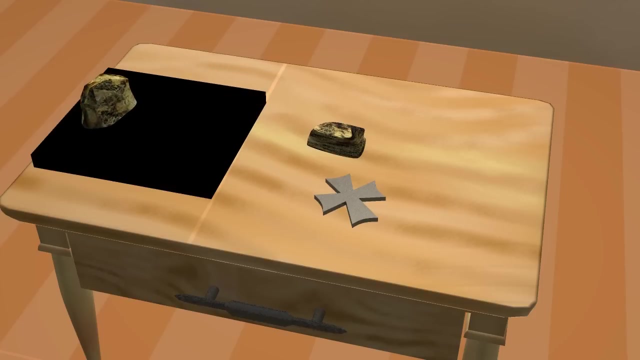 Becquerel prepared his experiment, as before, with a photographic plate coated with silver bromide emulsion and covered in the two thick sheets of black paper. He placed the potassium uranyl sulfate crystals on the plates, some directly on the black paper and others on top of various metallic objects. 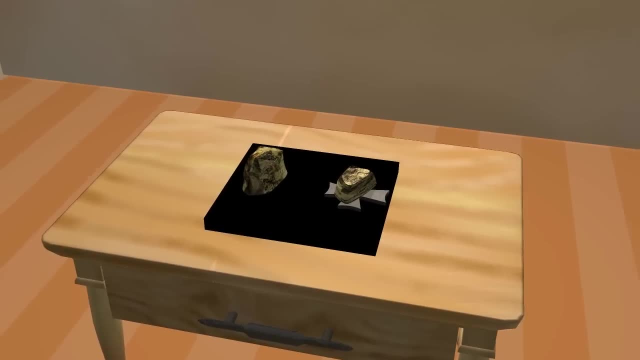 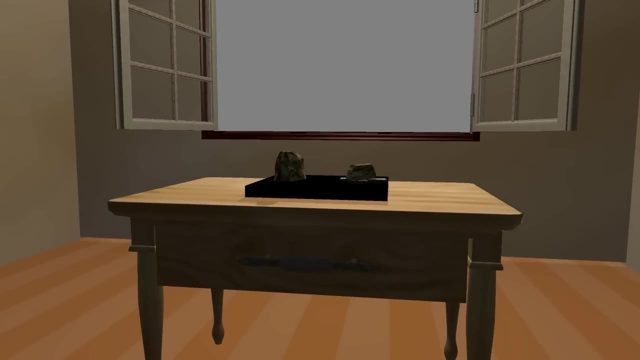 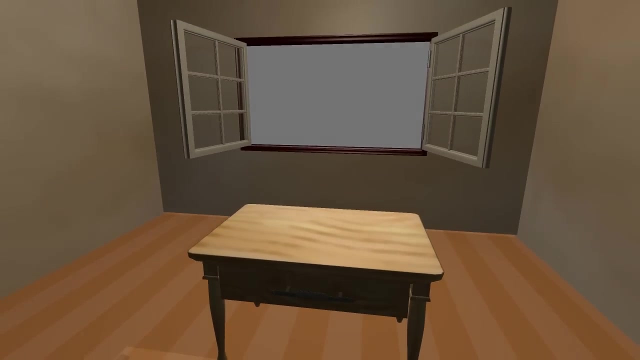 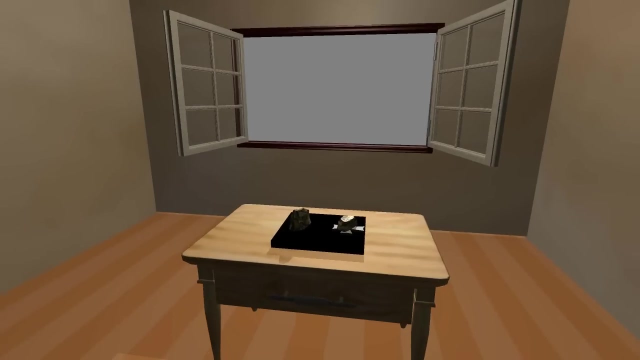 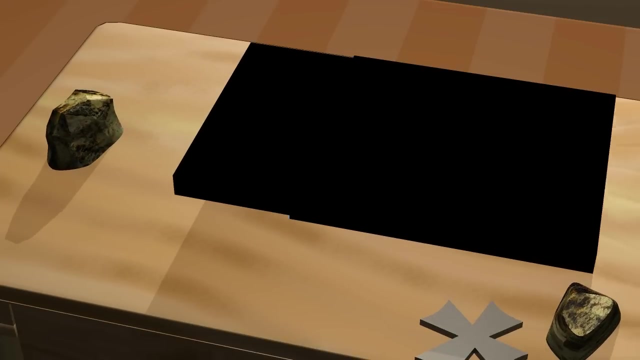 Since the skies were overcast, he placed the entire apparatus in a desk drawer, where it sat for the next three days. On that day, he developed the photographic plate, expecting at most a faint shadow from the phosphorescent stones. To his surprise, the silhouettes appeared with great intensity. 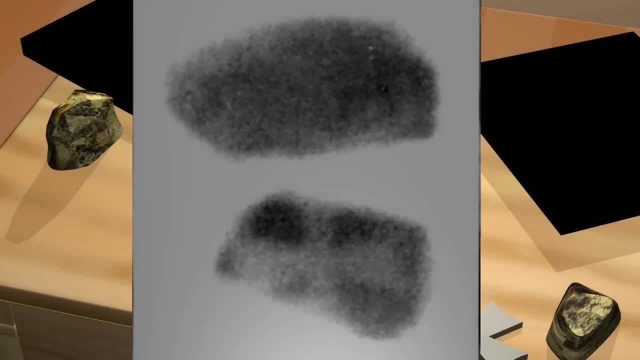 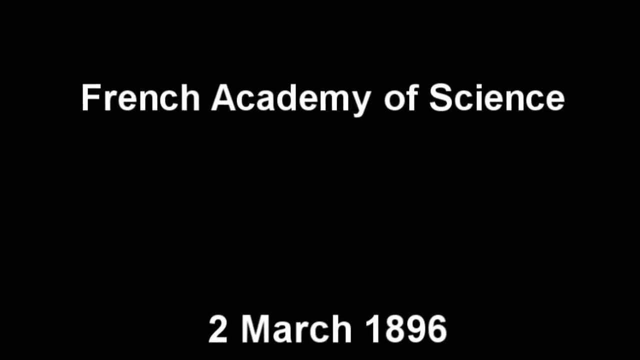 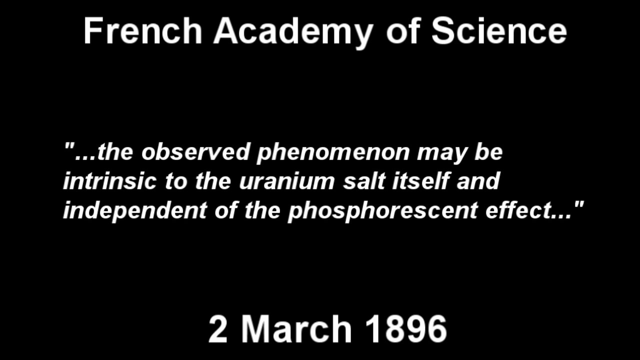 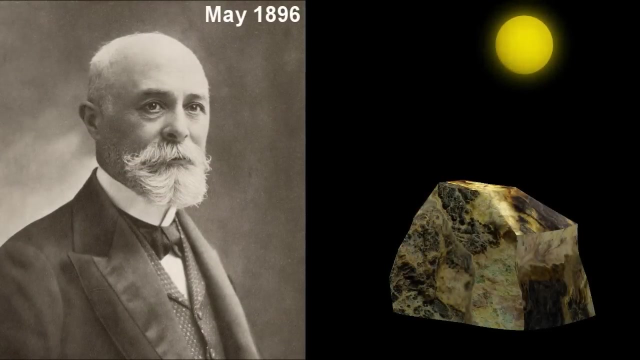 He immediately reported his findings to the French Academy of Science, suggesting that the observed phenomenon may be intrinsic to the uranium salt itself and independent of the phosphorescent effect. By May of 1896, after a number of experiments with non-phosphorescent salts of uranium, 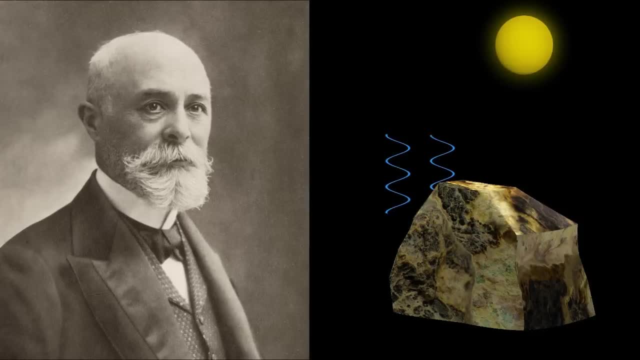 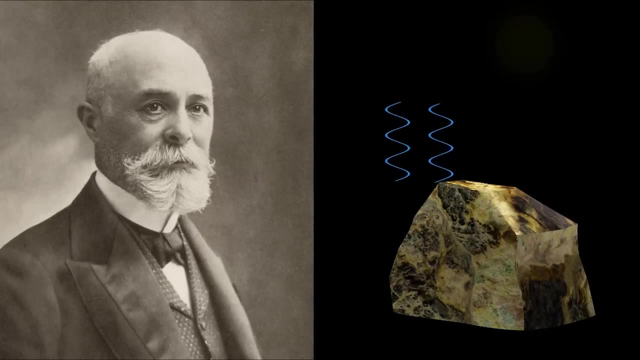 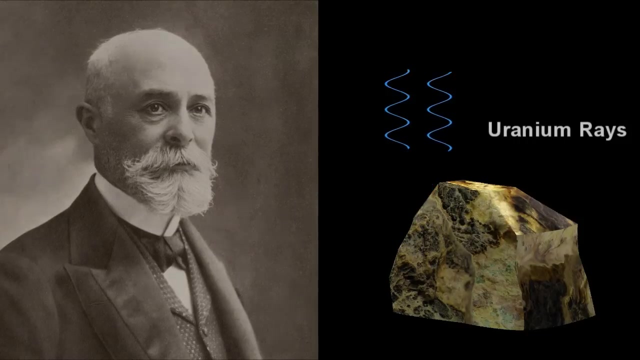 he arrived at the correct explanation that the penetrating rays were emitted spontaneously from the uranium mineral, without the need for an external source of energy or excitation by the sun. These became known as uranium rays. Maria Skłodowska-Curie, a native of the Kingdom of Poland in the Russian Empire, was 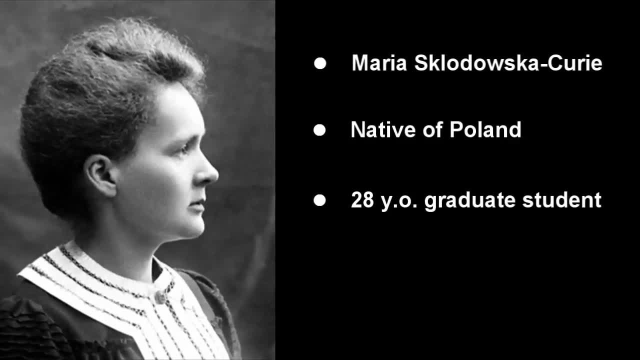 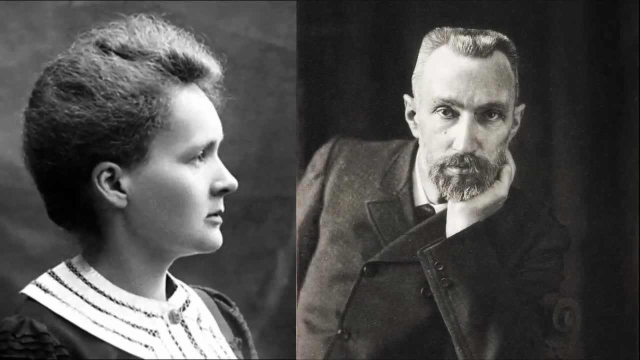 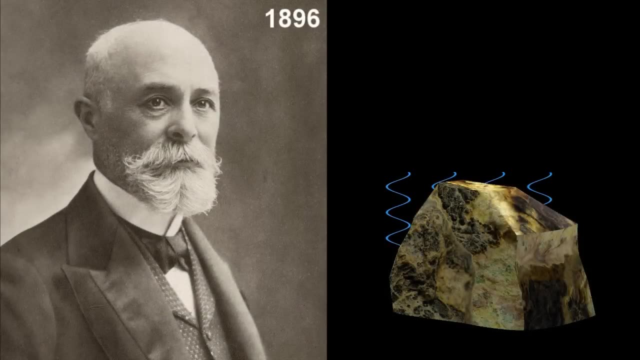 a 28-year-old graduate student of physics and math pursuing research on the magnetic properties of steel in her husband Pierre's laboratory at the Paris Municipal School of Industrial Physics and Chemistry when Becquerel announced his findings on uranium rays in 1896.. Soon after the birth of their first daughter, Irene, in September of 1897, Marie began looking. 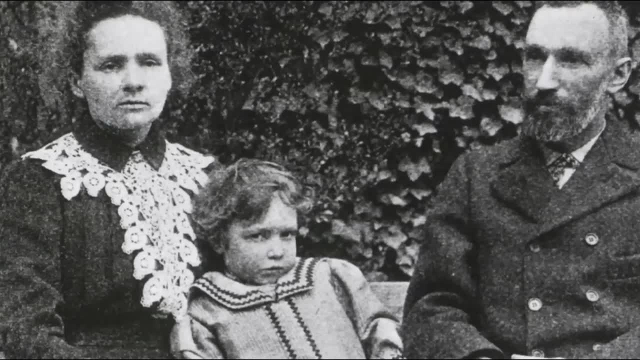 for a reason: to study the uranium rays. The discovery of the uranium rays in 1896 led to the discovery that the uranium rays were a research topic to pursue her doctoral degree in science. Familiar with Becquerel's discovery of uranium waves almost a year prior, she felt this would 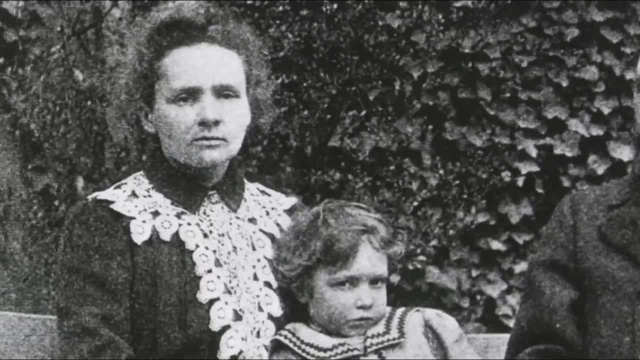 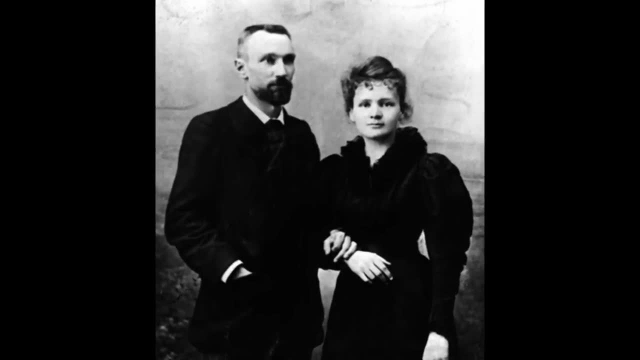 be a topic worthy of investigation, as there was so little existing research to review. As fate would have it, Marie's husband, of just over two years, was already a well-known scientist in Paris, as he and his brother, Jacques, shown here with their mother and father, had. 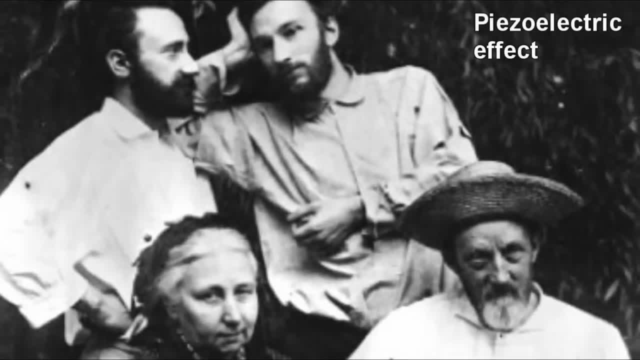 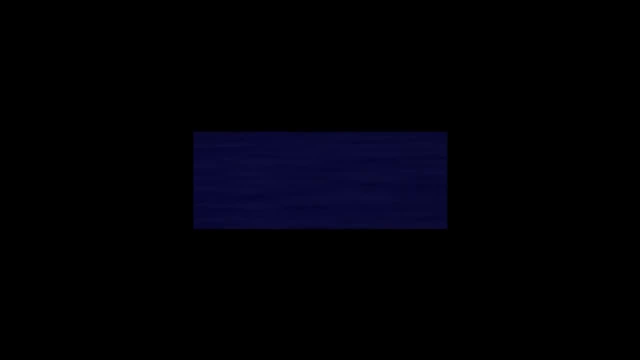 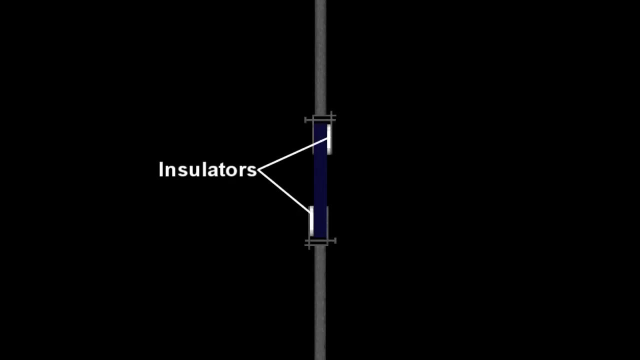 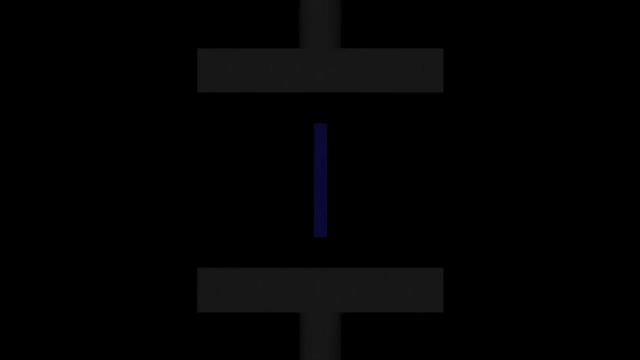 discovered the piezoelectric effect 17 years earlier. They demonstrated that…. …when certain crystals like quartz or Rochelle salt were deformed or compressed, the mechanical strain produced an electrical potential. They subsequently discovered the converse was also true, causing the crystals to deform. 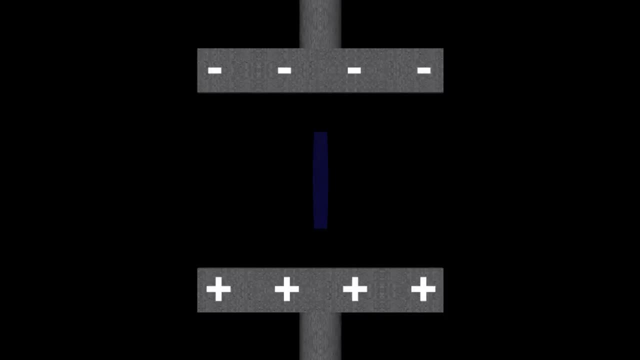 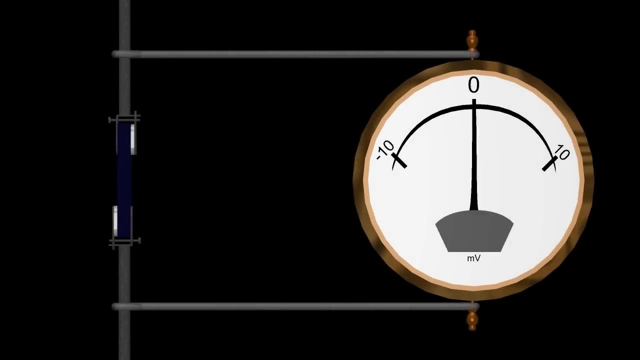 or compress when placed in an electric field. In fact, they noticed that compressing the crystal would produce a potential positive on one side and negative on the other, and that stretching the crystal would produce the opposite polarity. The brothers immediately put their discovery to practical use by inventing several pieces. 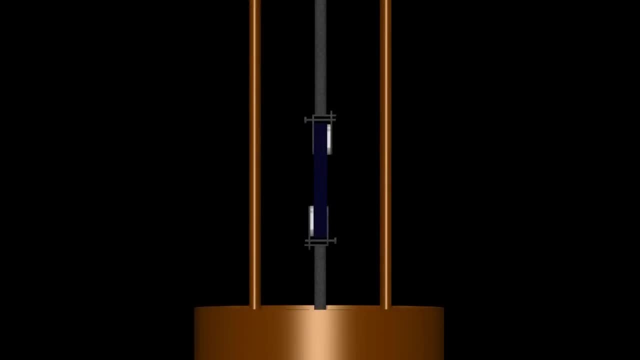 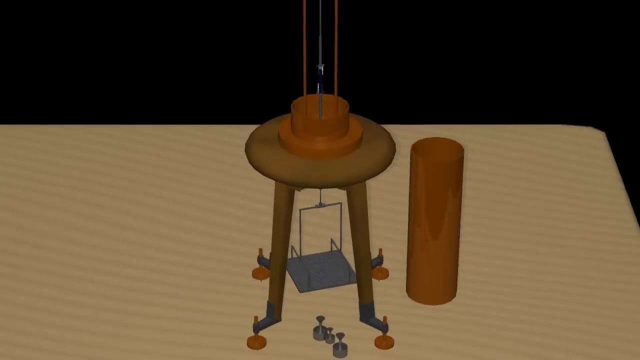 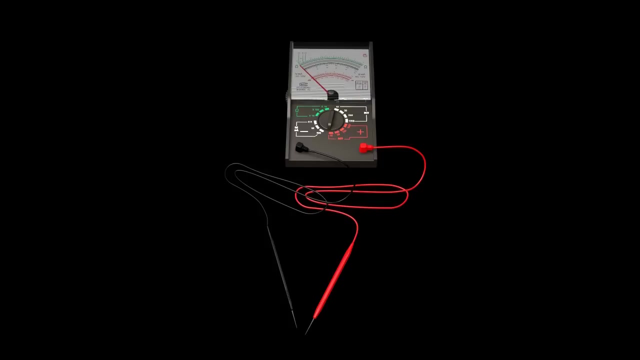 of sensitive laboratory equipment like this piezoelectric balance, capable of accurately measuring small quantities of material. Now, in 1880, the brothers would now be able to study the piezoelectric effect of the uranium and would not have had access to a modern-day voltmeter to carry out their experiments. 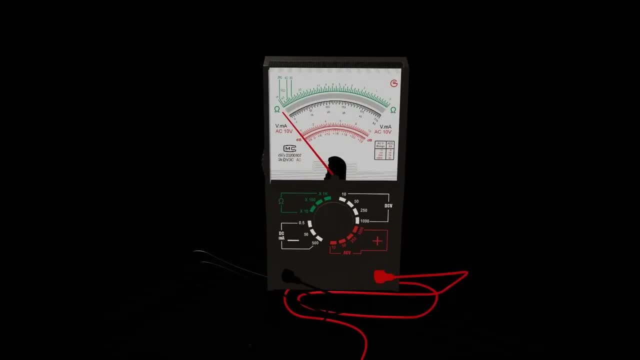 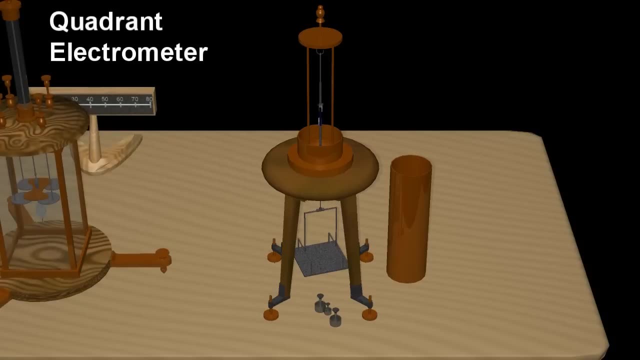 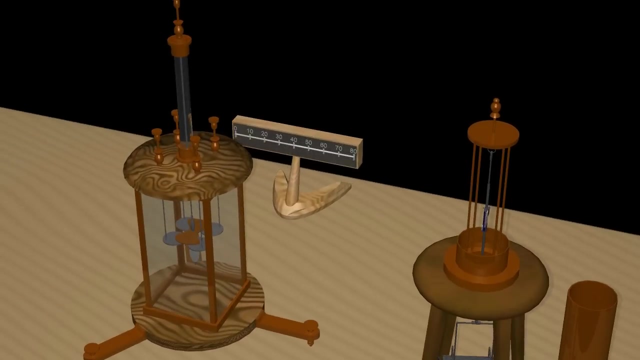 on the piezoelectric effect. At that time, the only instrument capable of accurately measuring electrical potential was an ingenious device called a Quadrant Electrometer, developed by Sir William Thomson or Lord Kelvin in 1857. The instrument consisted of a central torsion wire electrically isolated from the housing. 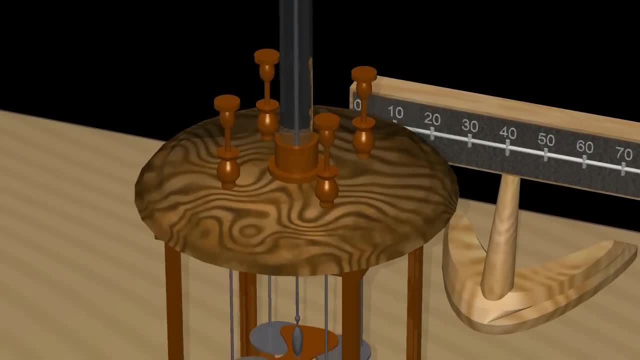 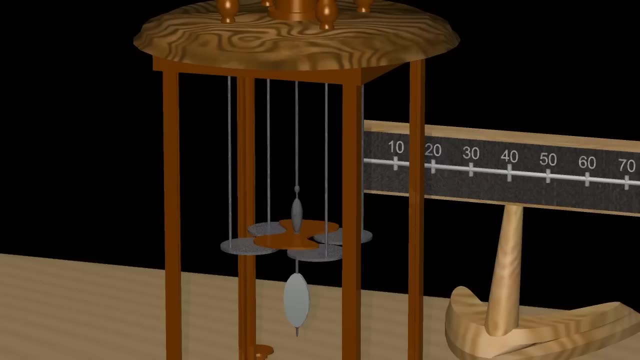 with four additional electrically isolated terminals, each with a special wire on the terminal, each of which communicated with one of four metallic plates suspended in the housing chamber. Just above the four plates, a metallic dumbbell-shaped vein was solidly affixed to the torsion wire. 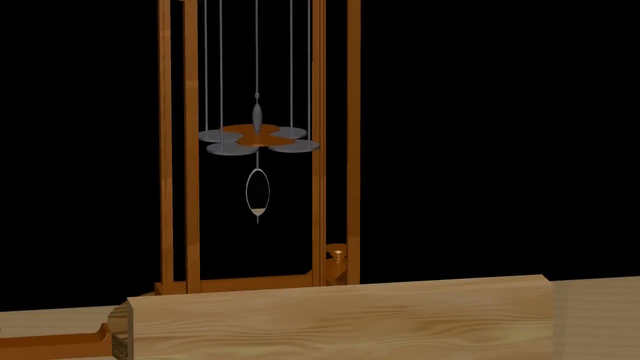 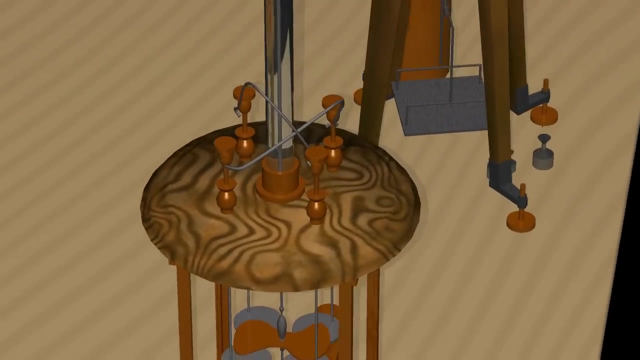 Below the plates and similarly affixed to the torsion wire, was a reflective mirror. Depending on the nature of the experiment, various wiring configurations could be utilized with the electrometer. Most commonly, the diagonal plates were electrically connected and the output leads from the test device were then connected to each of the diagonals. 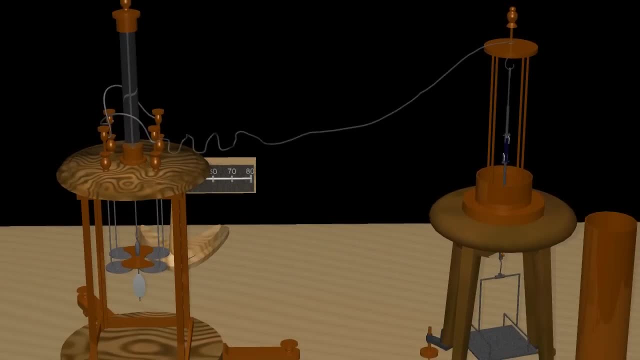 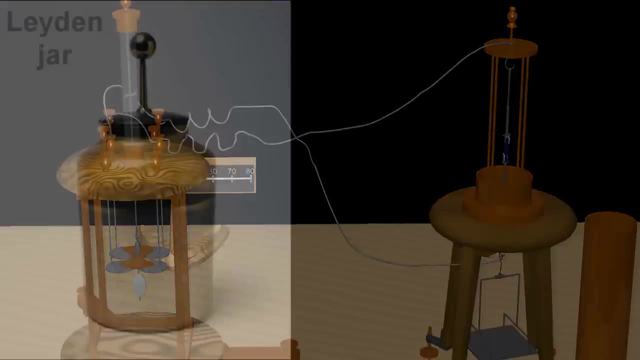 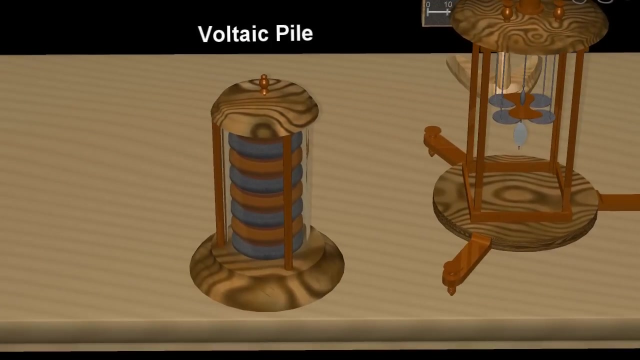 as shown. Finally, the lead to the torsion wire was connected to a voltage source such as a Leidenjar, precursor of the modern-day capacitor, or, as shown here, a voltaic pile or prototype battery, which consisted of alternating plates of copper and zinc separated by cardboard disks soaked. 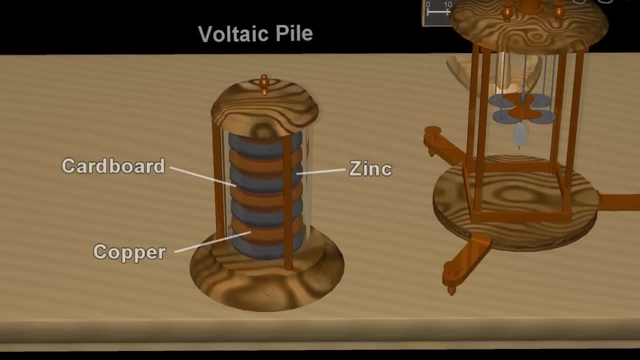 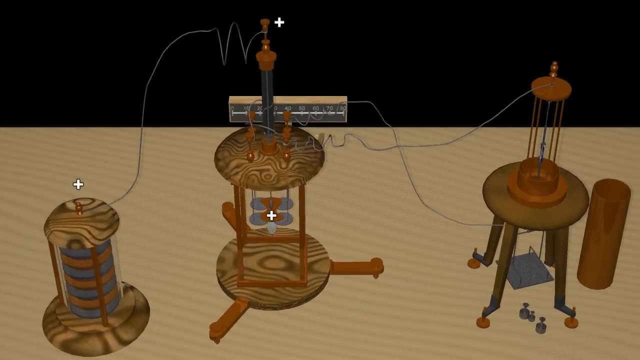 in salt water. This led to a positive charge on the electrical wires and dumbbell-shaped veins. The pile provided a positive charge on the torsion wire and dumbbell-shaped vane. As we weight the scale, the tension on the quartz crystal again produced a voltage potential. 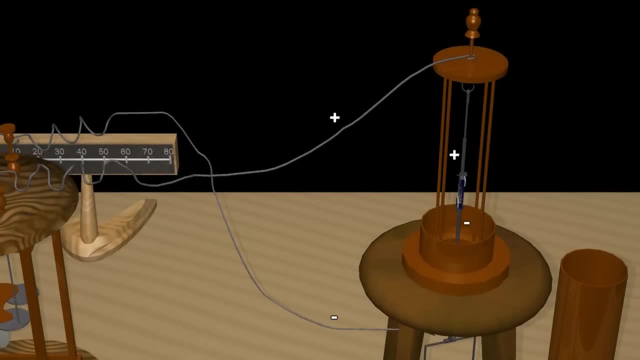 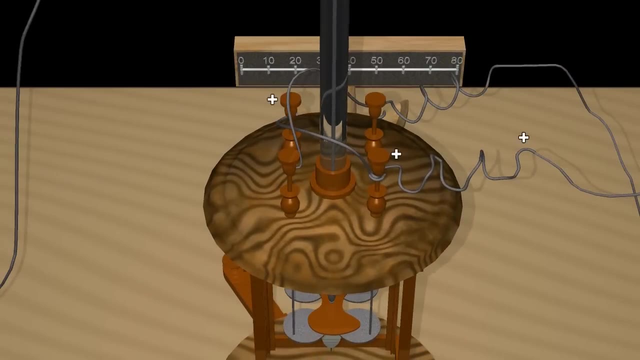 positive on one side and negative on the other, the strength of which is proportional to the amount of weight. The positive lead from the scale provides a positive charge to two of the four plates across the diagonal, and the negative lead puts a negative charge on the remaining two. 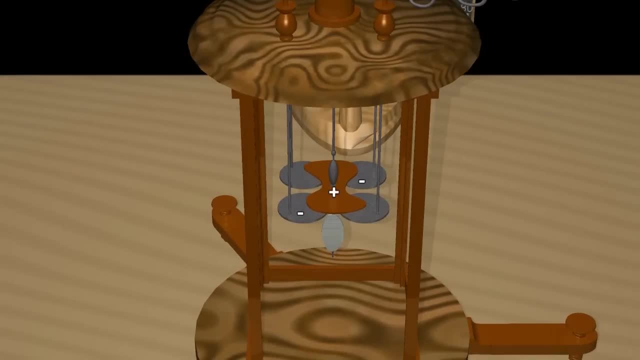 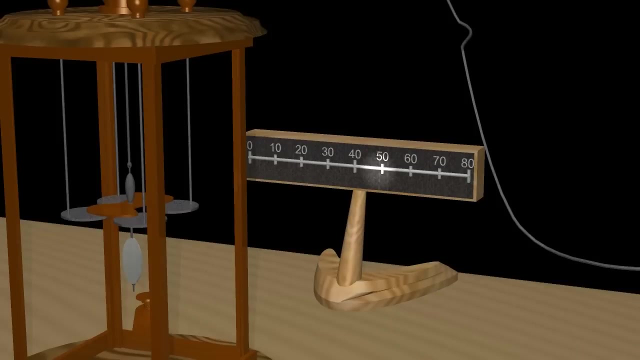 plates across the diagonal, Remembering that opposite charges attract and, like charges, repel. this configuration causes the tension wire to rotate as the vane is pushed away from the positive plates and pulled towards the negative plates. The reflective mirror rotates with the vane and wire and reflects a small light. 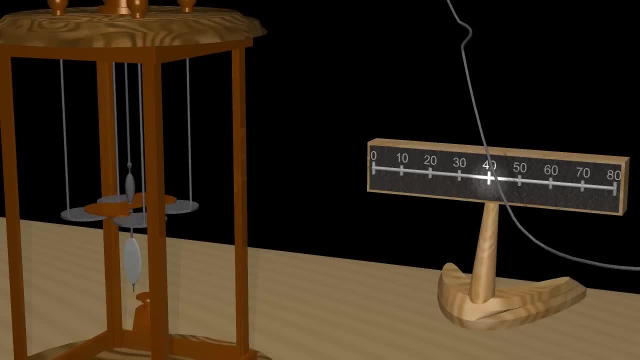 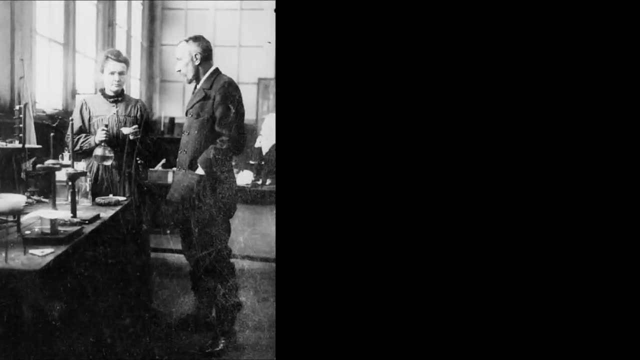 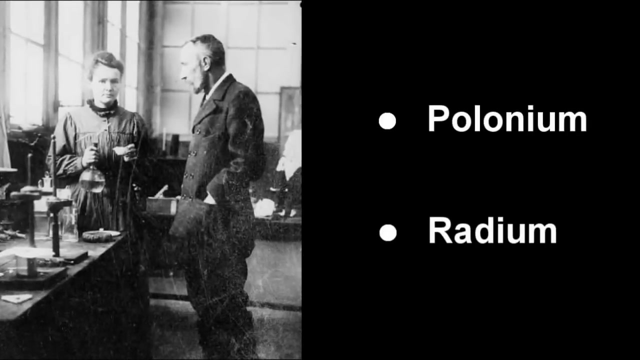 onto a scale board. The heavier the weight, the more rotation and the farther the light moves along the scale. Similar equipment, with some modifications, was instrumental in Marie's work in the subsequent discovery of the radioactive elements polonium and radium. nearly two decades later, Details of Marie's 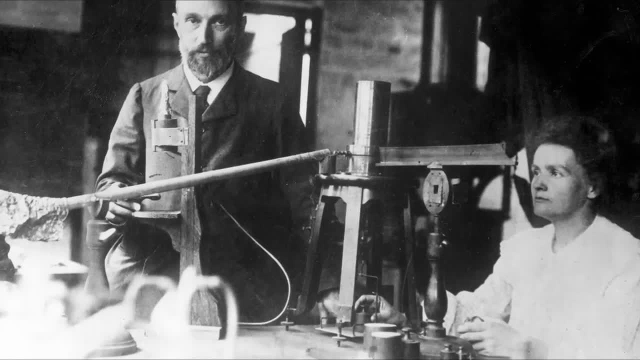 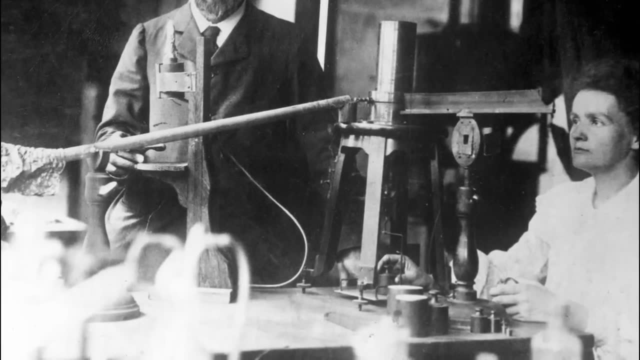 laboratory setup are surprisingly limited, and some of the descriptions I found are contradictory or nonsensical. This may be due to the fact that her notebook and many of her personal items are so radioactive that they are kept in lead-lined boxes in the National Museum of Art. 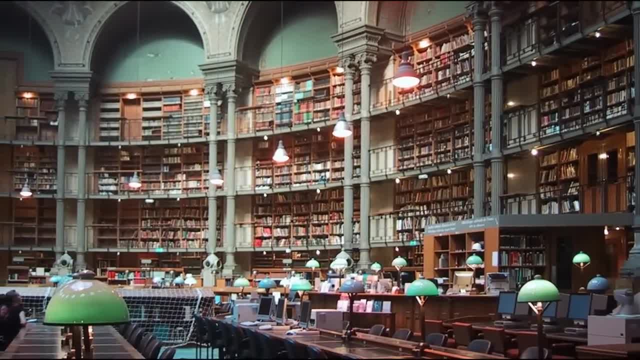 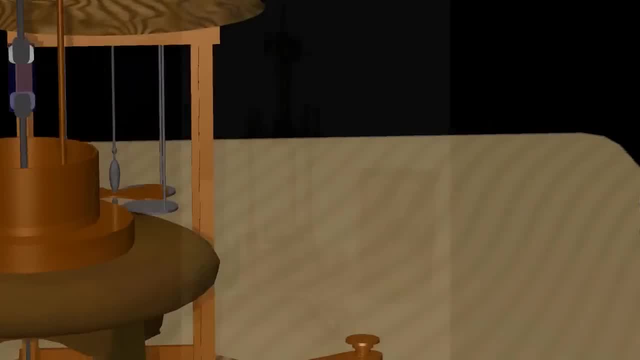 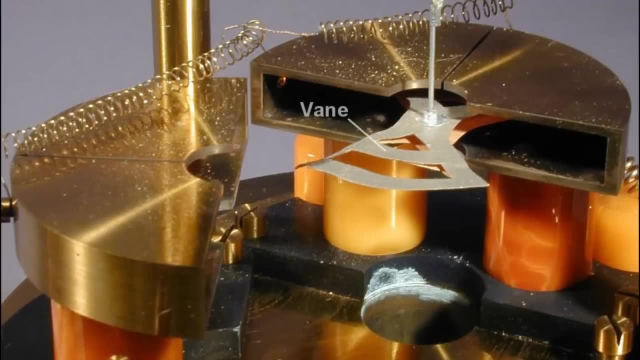 The National Library in France saw access as limited. The quadrant electrometer shown in the animation was probably not sensitive enough to carry out the Curie's work. This model, with the vane enclosed in a hollow cylindrical tube cut into quadrants, was likely the instrument of choice. 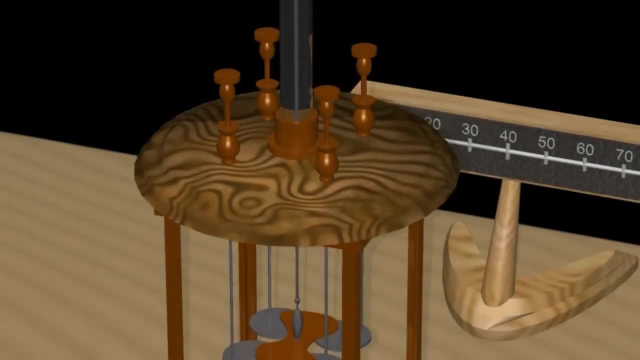 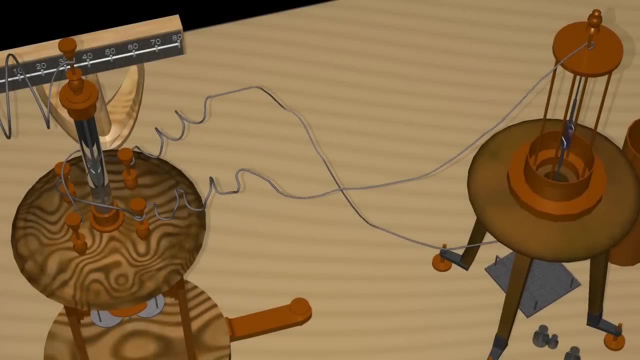 For demonstration purposes. we'll continue to use the earlier model. however, The electrometer requires some rewiring as well. We're going to switch the leads, placing the positive on the front terminal and the negative on the back. We'll also remove the diagonal electrical connections on the terminals. 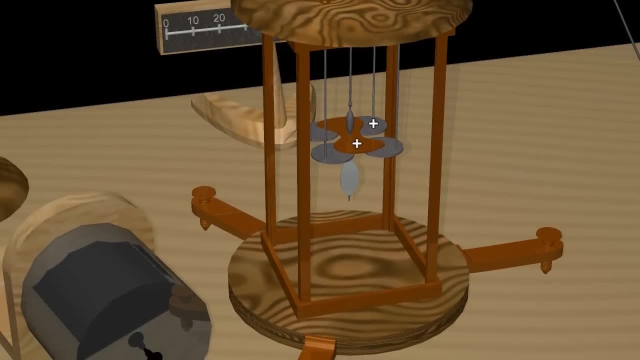 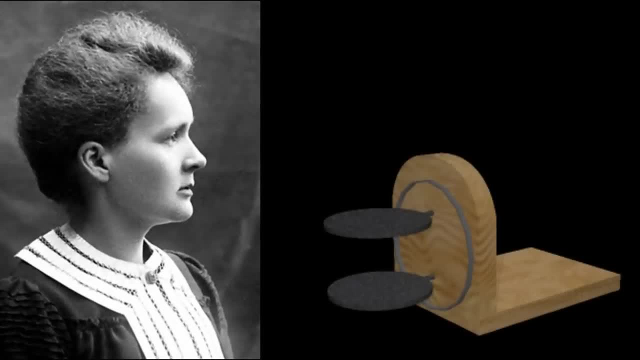 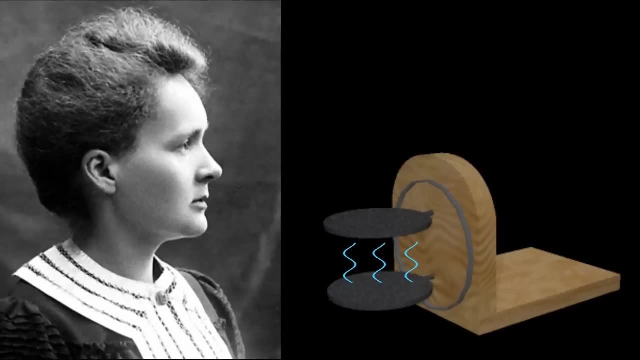 This configuration applies a positive charge to the front right plate and the left plate to the left. direct physical connection. Marie assumed that the effect of uranium waves on the conductivity of air between the condenser plates was similar to the action of radio waves, and thus coined the term radioactivity to describe the. 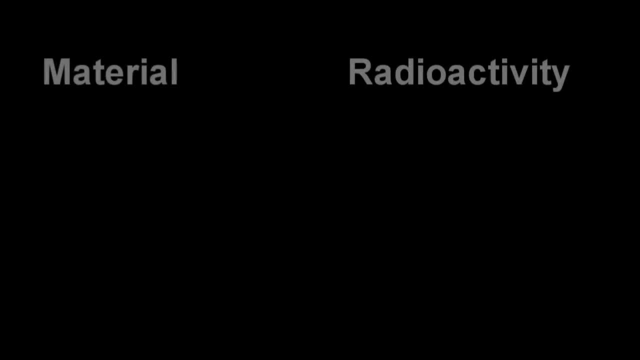 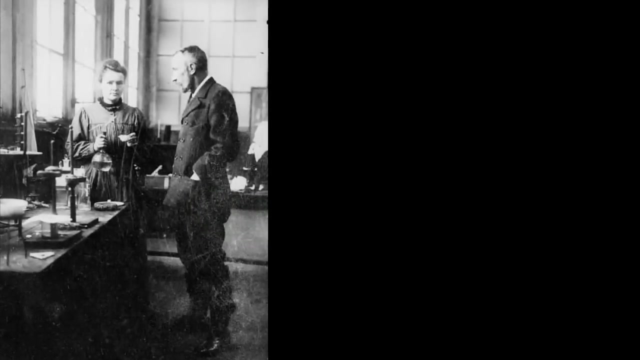 observed phenomenon. Marie correctly postulated that the intense radioactivity of the pulverized pitch blend could not be explained by the uranium content itself and therefore other active elements were likely present in the mineral. She and her husband began a systematic search to isolate these elements, finding initial success in July 1898 with the 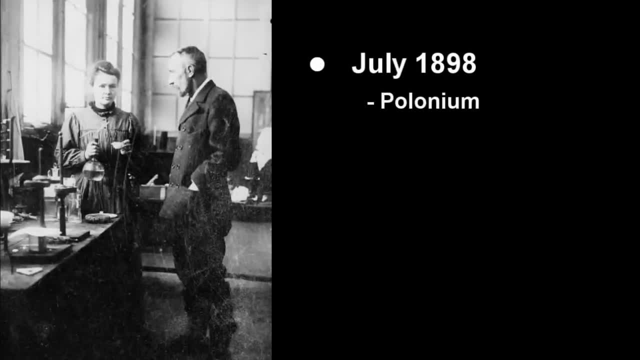 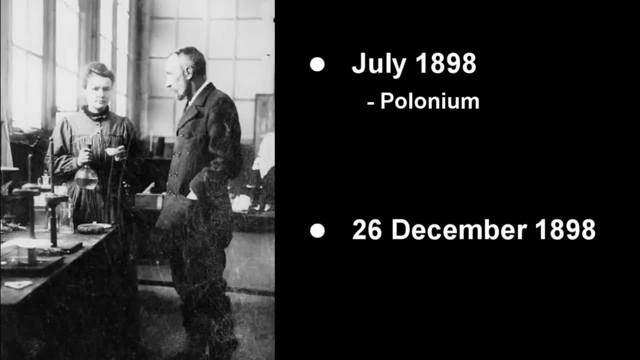 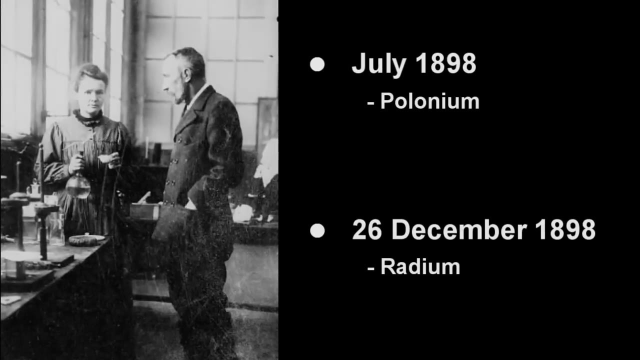 announcement of a new radioactive element, polonium, named after Marie's homeland, Poland. On 26 December of 1898, the Curies announced the discovery of their second isolated radioactive element, which they named radium, after the Latin word for ray, In 1899,. 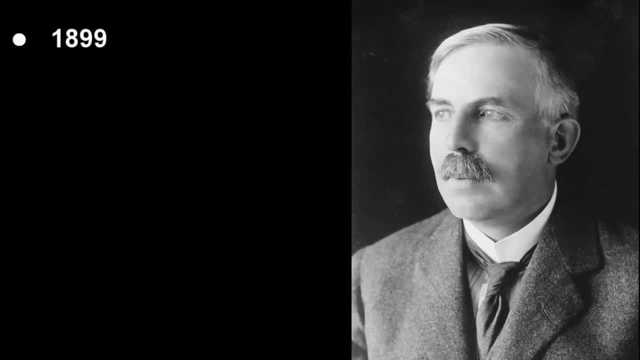 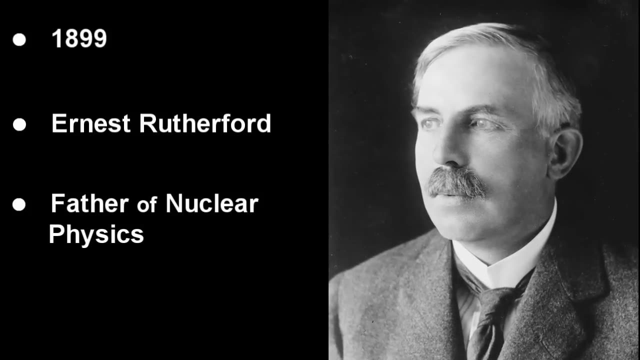 within one year of the Curies announcing their discovery of the new element radium, Ernest Rutherford, the father of nuclear physics also working with uranium minerals, announced his discovery of two different types of radioactivity that seemed to differ in their penetrating power when compared to the 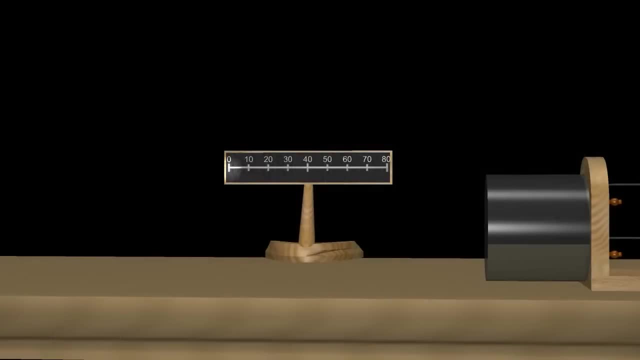 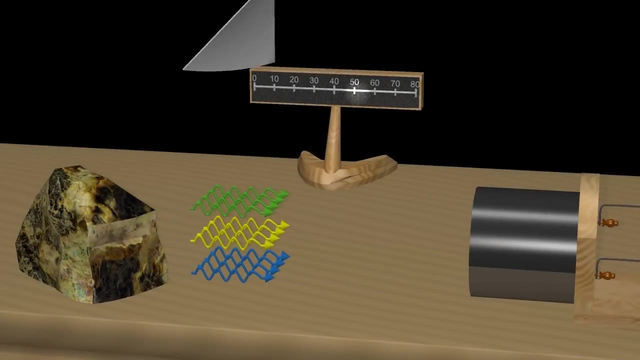 previously discovered x-rays. The first of these radiations, which he labeled alpha, were blocked by a sheet of paper. The second, labeled beta, passed through the paper but were blocked by a thin sheet of metal foil. The radiation that passed through the paper and the foil initially remained. 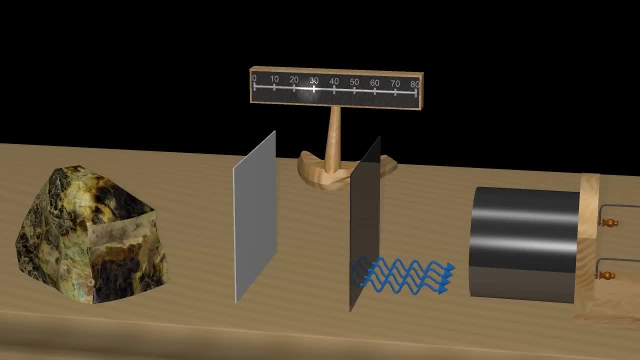 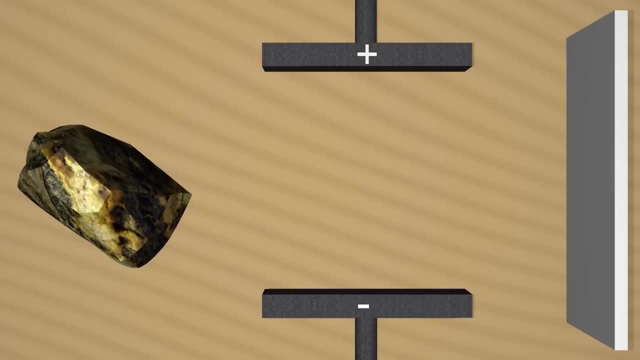 unnamed. Subsequent studies by Rutherford and others showed that the previously labeled alpha radiation moved relatively slowly and exhibited a small deflection in electric field towards the negative polarity. Beta radiation, on the other hand, moved much faster and showed a large deflection to the positive pole of. 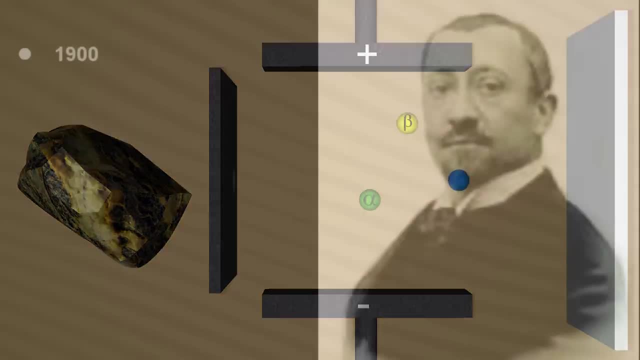 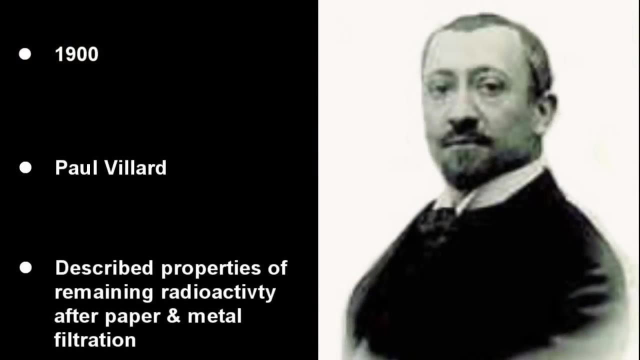 the same electric field. A year later, in 1900,, the French physicist and chemist Paul Villard described the remaining rays, reiterating their presence in the light, their ability to penetrate thick sheets of metal and showing no deflection in an electric. 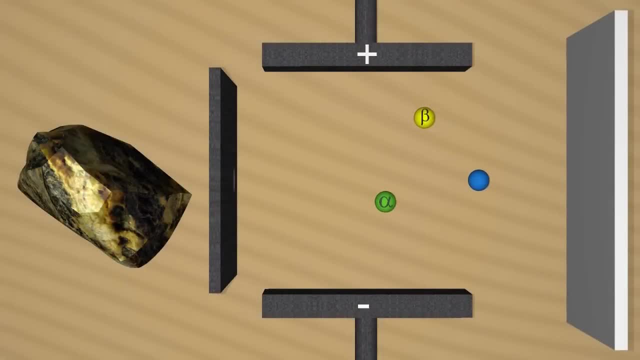 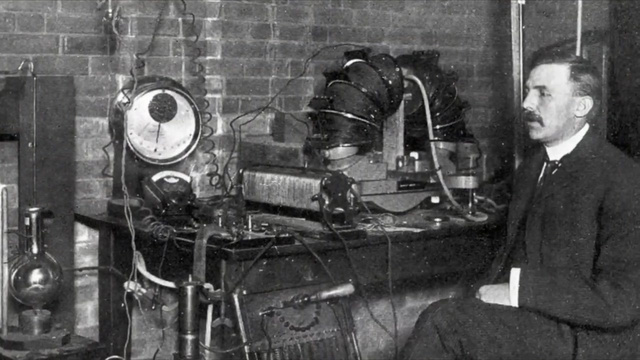 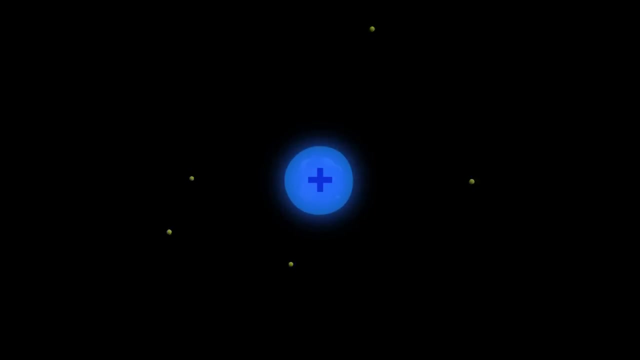 or magnetic field. Rutherford eventually named these rays gamma in 1903.. Rutherford's investigations over the next decade on radiation and matter led him to the now generally accepted conclusion in 1911 that atoms consisted of a small positively charged nuclei surrounded by a large empty space encircled by tiny negatively charged 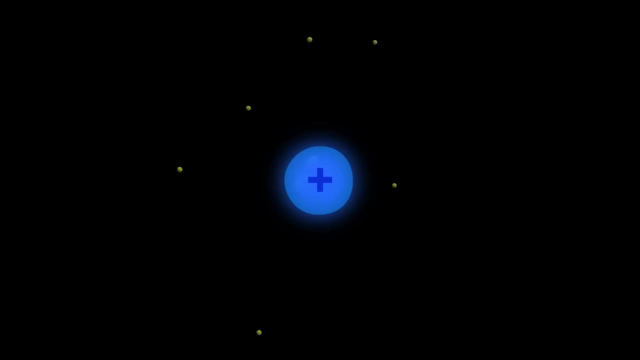 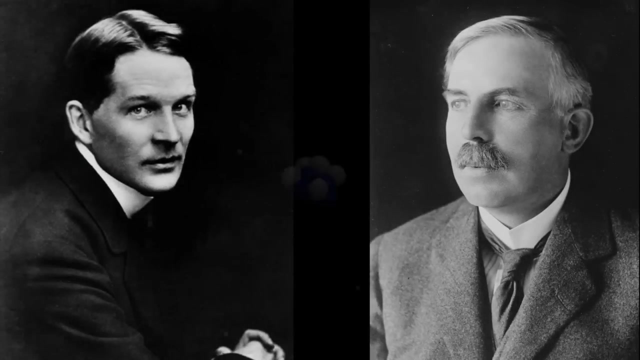 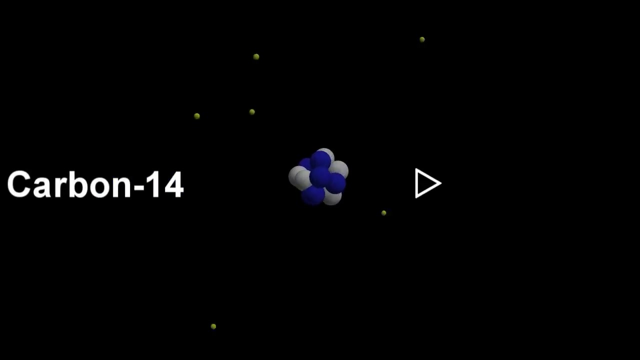 electrons. In collaboration with Frederick Soddy, he was the first to correctly suggest that radioactive phenomenon was an atomic process due to the spontaneous disintegration of the atom and transmutation of elements into completely new substances. The two also suggested the phenomenon was an atomic process. 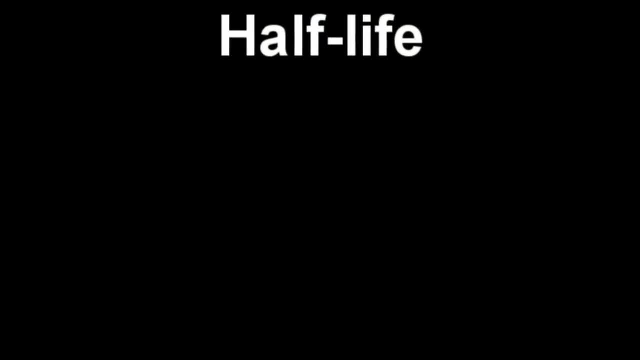 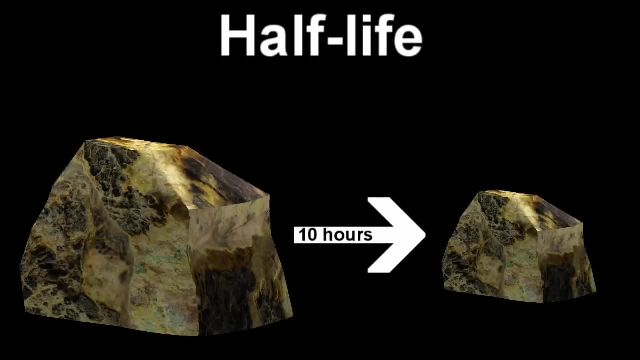 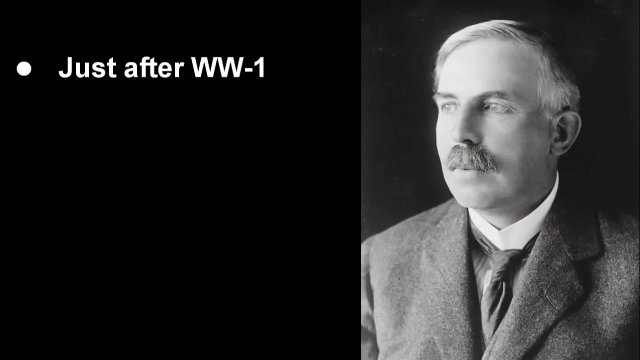 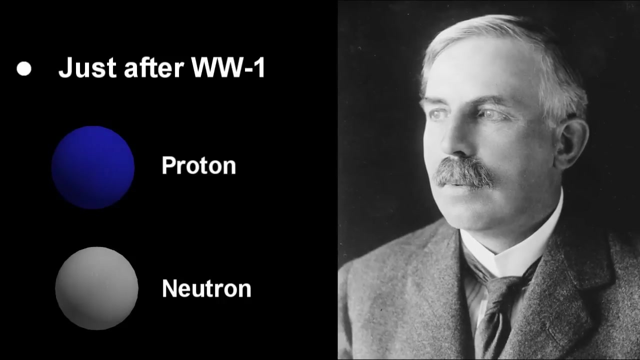 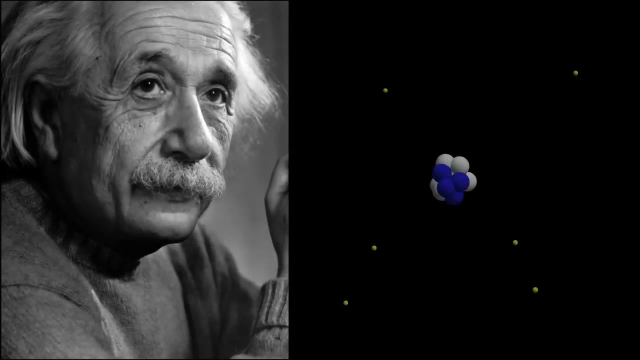 Rutherford is credited with the discovery of the proton and at the same time suggested the existence of the neutron, the two components of all atomic nuclei. Rutherford's model of the atom, along with other theories like general relativity, now provide us with an accurate and relatively simplistic. 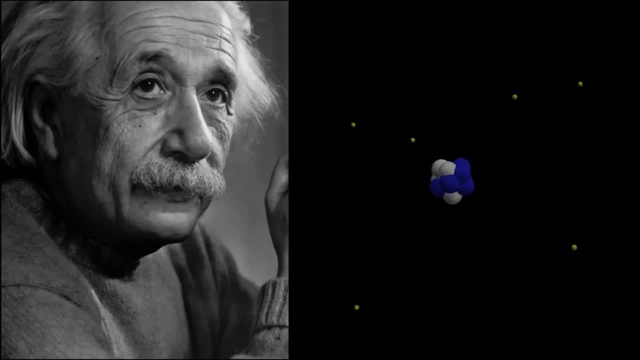 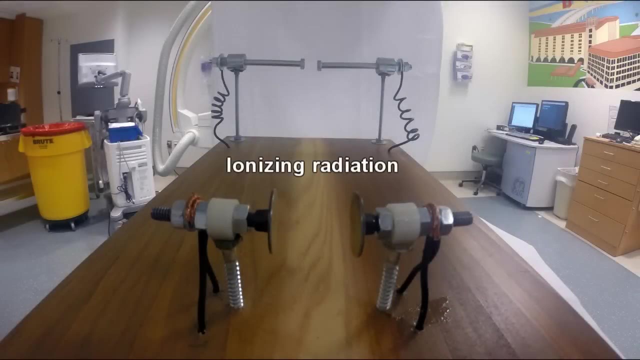 explanation of all radioactive phenomenon. This apparatus is designed to explain the concept of ionizing radiation. A high voltage power source provides a 300,000 volt potential at the two sets of terminals which are connected in parallel. The rear terminals are a fixed distance apart and the front terminal distance is adjustable. 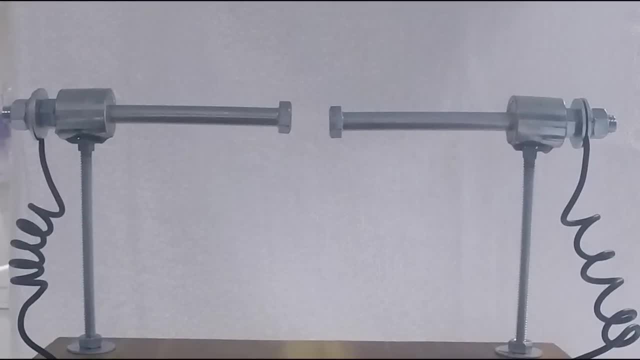 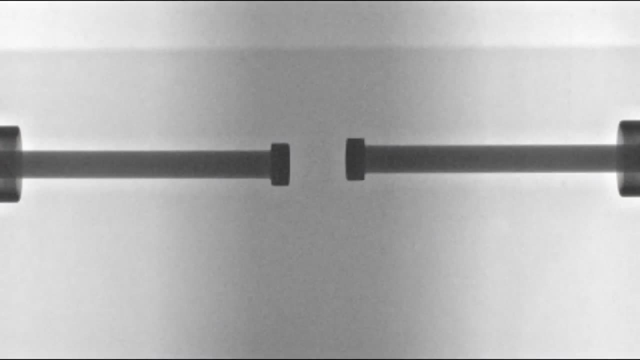 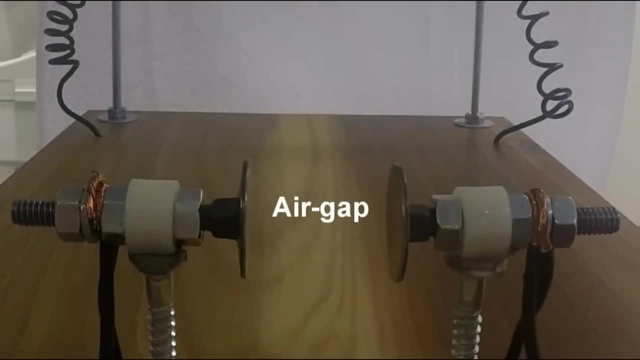 Ordinarily, air is a poor conductor of electricity. However, a spark will jump an air gap if the terminals are close enough and the voltage is sufficient to push the electrons across the gap. In addition, the spark will take the path of least resistance, so if the front terminals 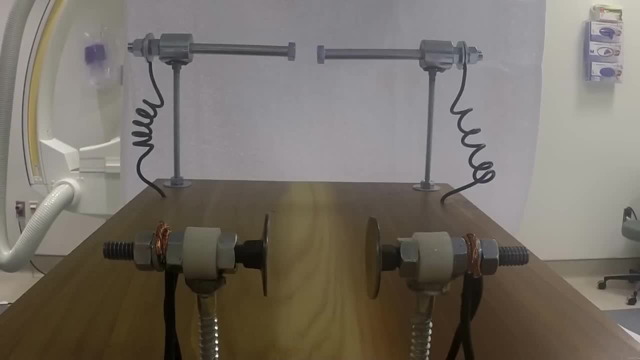 are closer together than the rear, the spark will not be able to push the electrons across the gap. In addition, the spark will take the path of least resistance. so if the front terminals are like an air Poor, If we then move the front terminals apart until their distance just exceeds that of 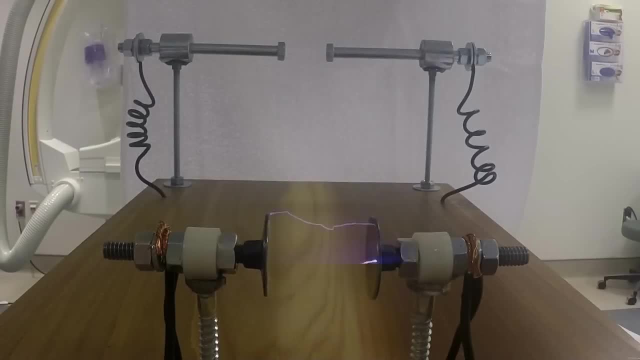 the rear terminals, the spark jumps the later gap. Now, if we turn on our fluoroscope and maintain the front terminal distance, the spark moves from the rear fixed terminals to the front terminals, even though they are further apart. When we turn the radiation source off, the spark again takes the path of least resistance. 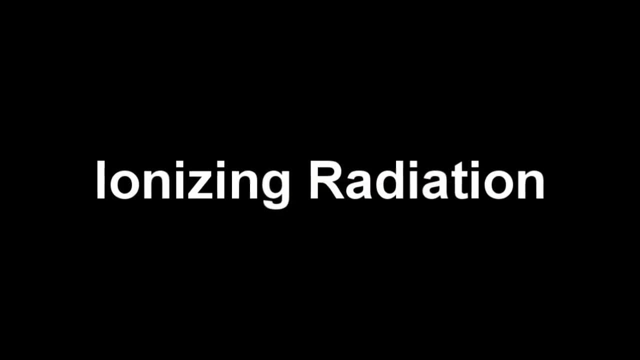 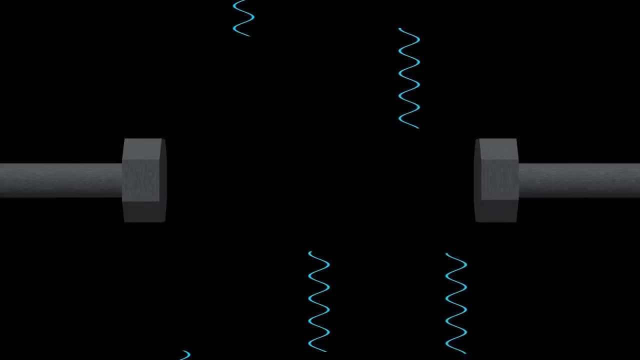 resistance to the rear terminals. This demonstrates the phenomenon of ionizing radiation. When the X-rays, a form of ionizing radiation similar to gamma rays, pass through the air gap between the front terminals, they can knock away some of the orbiting electrons around the nuclei. 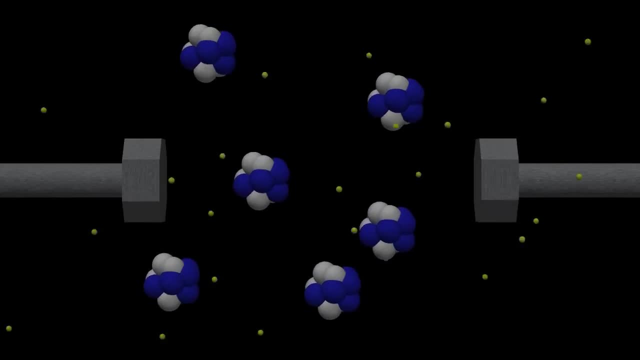 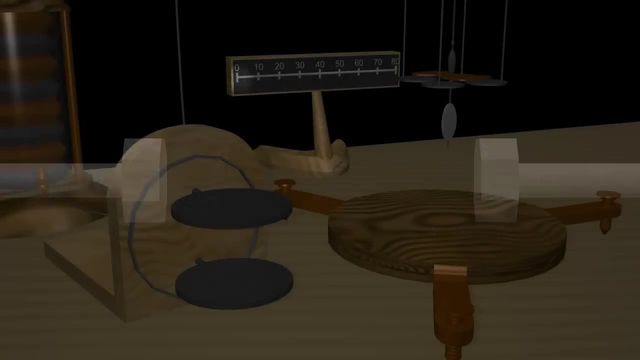 of the oxygen, nitrogen and other gases in the air, turning neutral atoms into positively charged ions. These ions reduce the electrical resistance between the larger gap and allow a spark to jump across the terminals. This is the same phenomenon Madame Curie noted in her 1897 and 1898 experiments describing the increased conductivity of air produced. 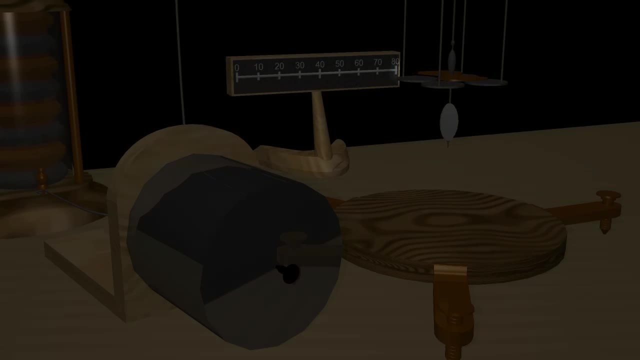 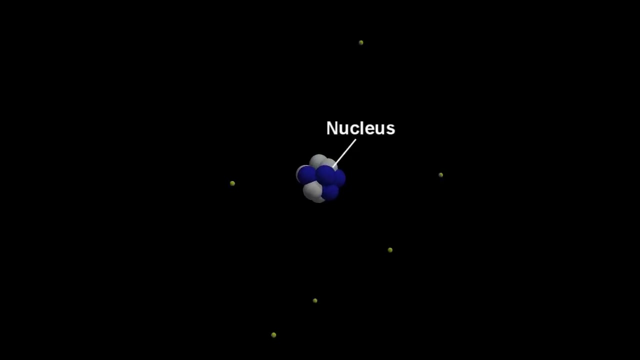 by uranium waves. As suggested by Rutherford, the atom consists of a central nucleus containing a mixture of the subatomic particles, the positively charged protons and the neutral neutrons. Encircling the nucleus are the negatively charged electrons. The relative mass of these subatomic particles are as follows: 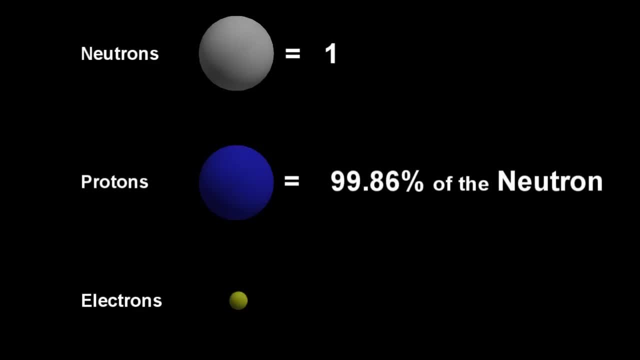 Neutron 1. Proton: 99.86% of the neutron. Electron: 0.054% of the neutron. As you can see, most of the atomic mass of the element is attributable to the protons and neutrons in the nucleus, with a negligible contribution from the encircling electrons. 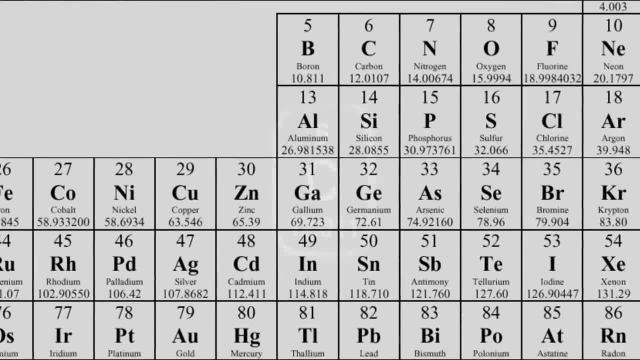 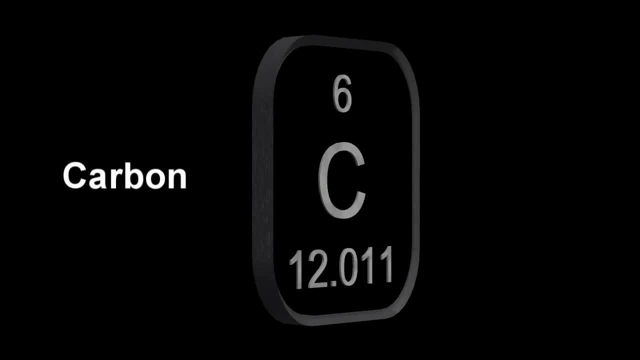 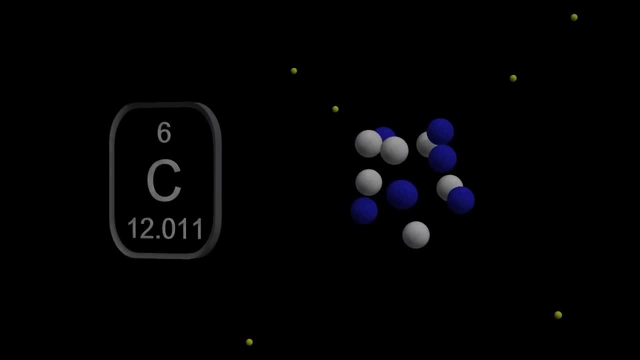 When we look at an element on the periodic table, the central letter represents the chemical symbol or abbreviation, in this case the basic building block of all life on Earth, the carbon atom. We'll explode out the nucleus slightly so we can easily count the components. 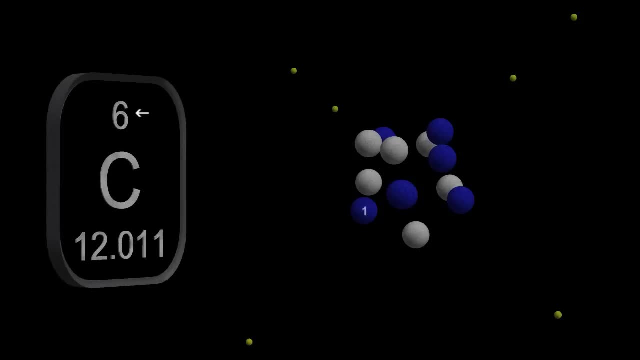 The upper number above the chemical symbol describes the number of protons in the nucleus and is called the atomic number. The lower number is the atomic mass and accounts for the total mass of the atom, including all the protons and neutrons in the nucleus and the 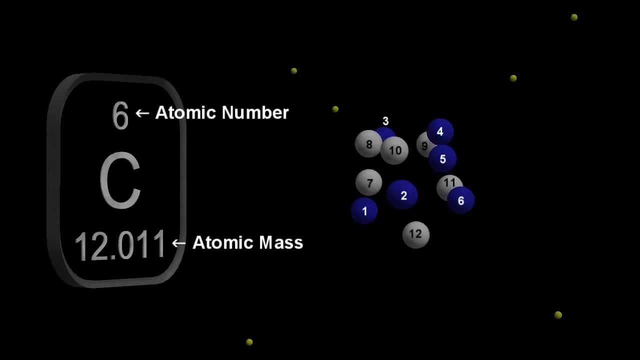 minuscule contribution from the encircling electrons. The chemical behavior of an element is determined by the number of encircling electrons, and to maintain electrical neutrality, there are always the same number of protons in the nucleus as there are orbiting electrons. Therefore, the chemical identity is determined solely. 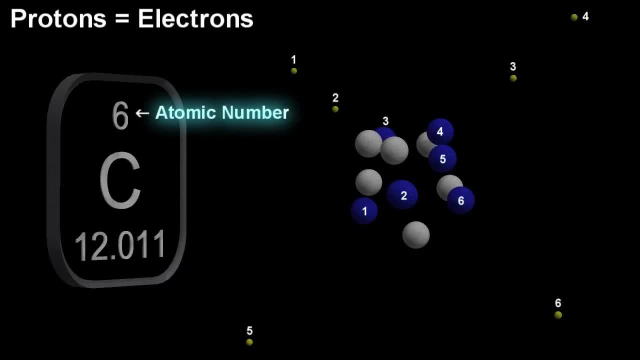 by the atomic number. Increasing or decreasing the number of neutrons in the nucleus creates isotopes of that element and changes the atomic mass, but does not affect the chemical behavior. For instance, if we add 2 neutrons to the nucleus of the carbon atom, the atomic number 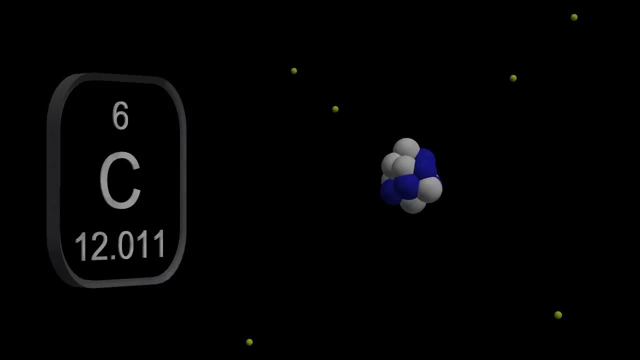 remains unchanged at 6, but the atomic mass increases by 2 to 14.. Some may recognize carbon-14 as the unstable isotope of the carbon atom used in carbon dating of ancient archeologic and geologic artifacts, With a half-life of approximately. 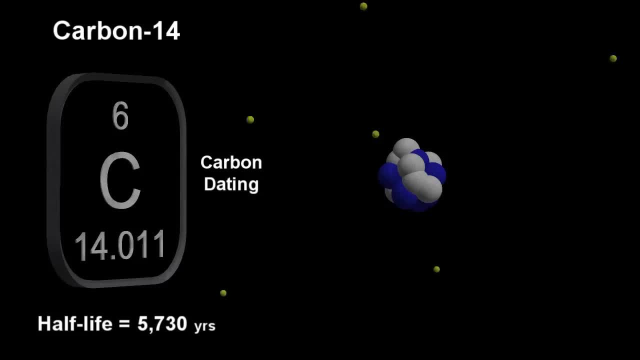 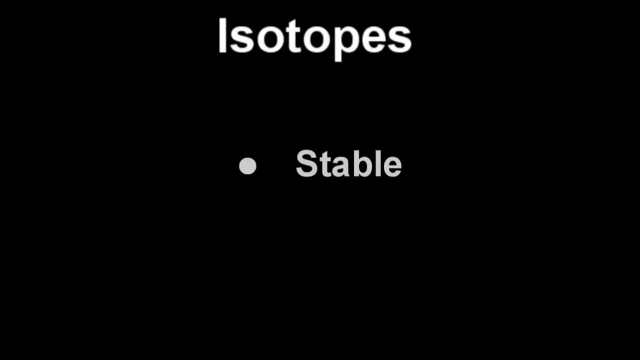 5,730 years. this methodology can be used to confirm the atom behavior and the cosmic energy potential in the nucleus. This methodology can be used to determine the age of artifacts up to approximately 50,000 years old. Some isotopes are stable and some are unstable. 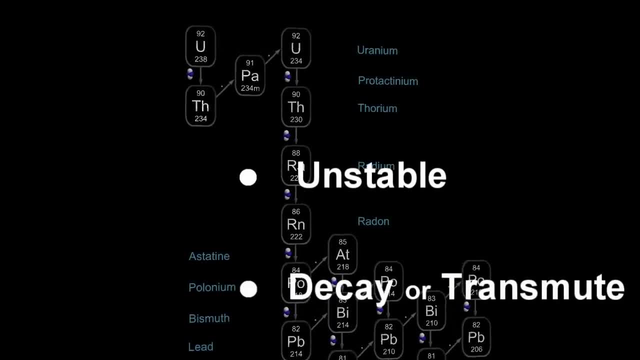 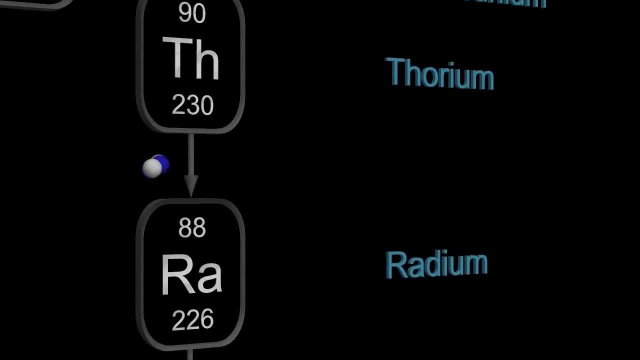 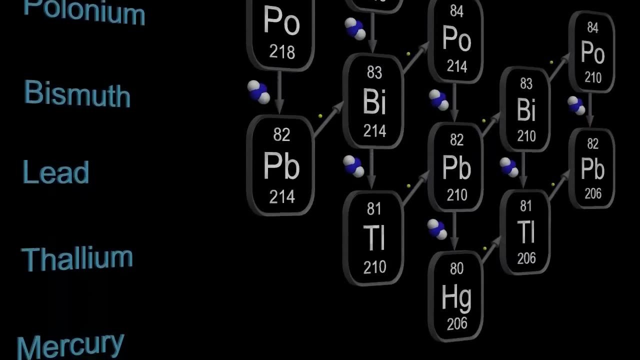 The unstable variety can decay or transmute into different elements that themselves may be stable or unstable. With enough time, all unstable isotopes will eventually transmute into stable elements through a decay chain, as shown here with uranium-238, eventually becoming the stable element lead over billions of years. 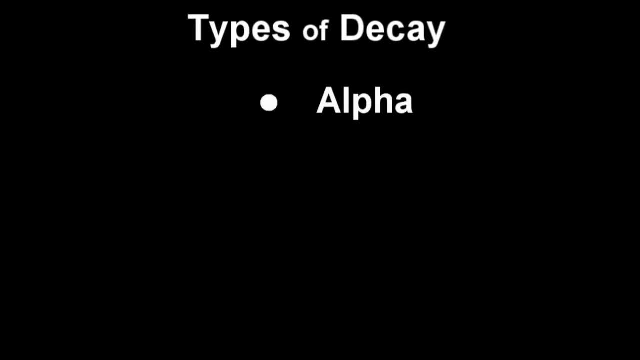 A variety of nuclear decay processes exist, but we will discuss the three most common in one special situation. It may be useful to pause the video at this point and print out a copy of the periodic table to use as a guide for the following discussion. 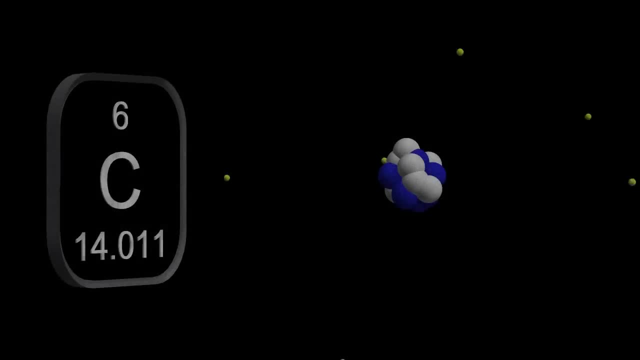 Using our carbon-14 isotope, we've already determined that we have too many neutrons compared to our stable carbon-12 nucleus. This particular isotope decays by one of the neutrons, giving off a small negatively charged particle or electron, just like the electrons encircling the nucleus. 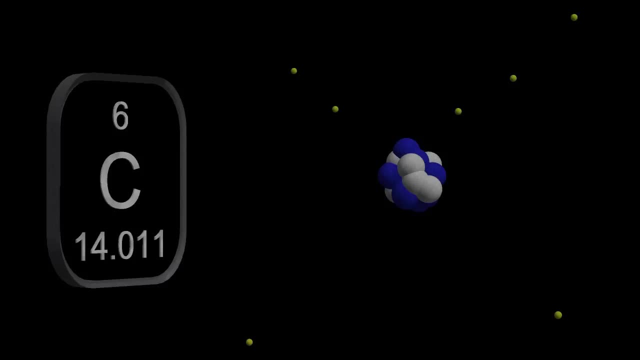 and leaving behind a proton. In addition, to account for an apparent loss of momentum and energy in the transformation, a theorized small neutral particle called an antineutrino is also released: The neutrino and its antiparticle, the antineutrino. 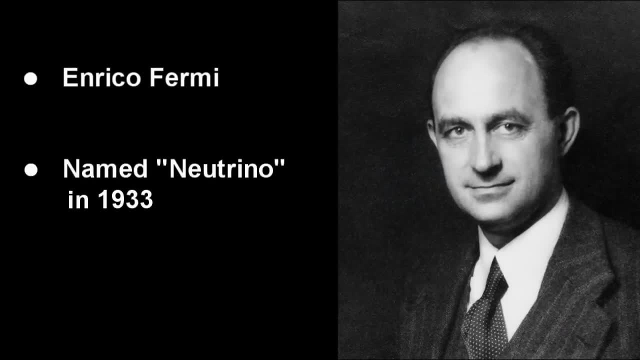 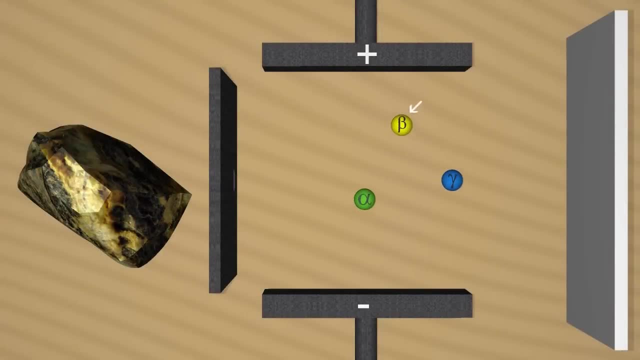 were named by the Italian physicist Enrico Fermi in 1933 and literally translates as little neutral one. The negative electron that is given off would of course move toward the positive pole of an electric field and corresponds exactly to the beta type radiation described by Rutherford in 1899.. 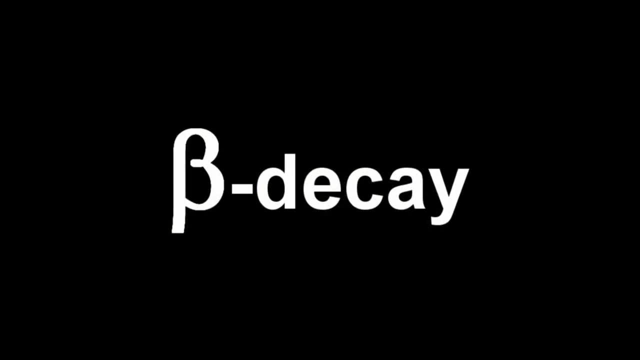 Therefore, this type of decay is referred to as beta decay. More specifically, this is beta minus decay, since the small electron released is negatively charged. You'll see why we make this distinction in a moment. If we look at our chemical placard, 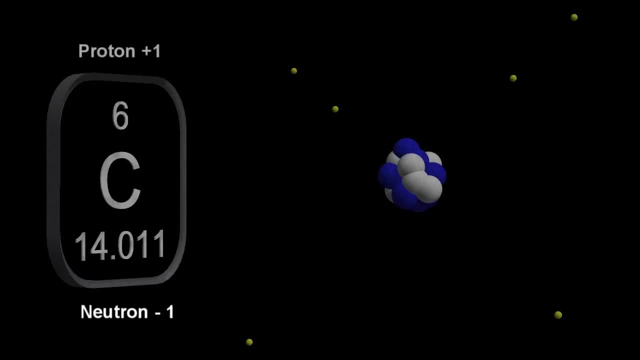 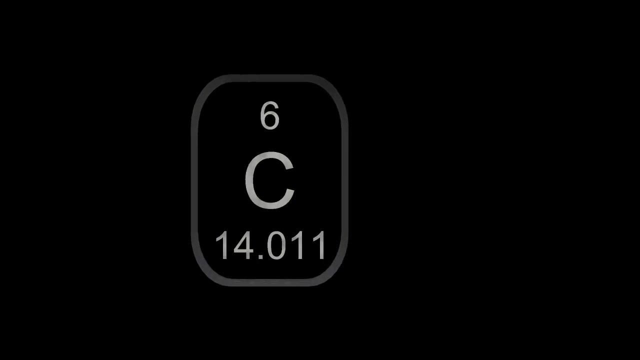 our carbon atom has now lost one neutron and gained one proton. Therefore, our atomic number goes up by one and our atomic mass is basically unchanged. Looking at our periodic table, the element corresponding to this configuration is nitrogen and is stable. Therefore, carbon-14 transmutes to stable nitrogen. 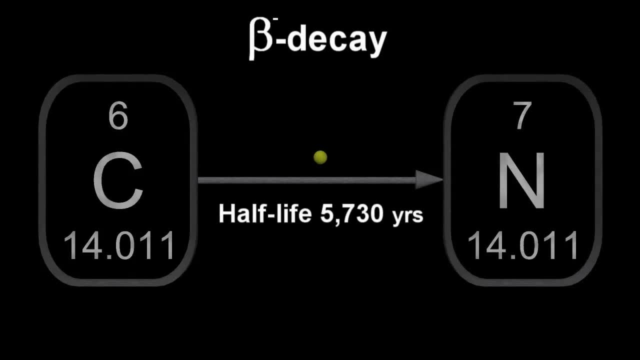 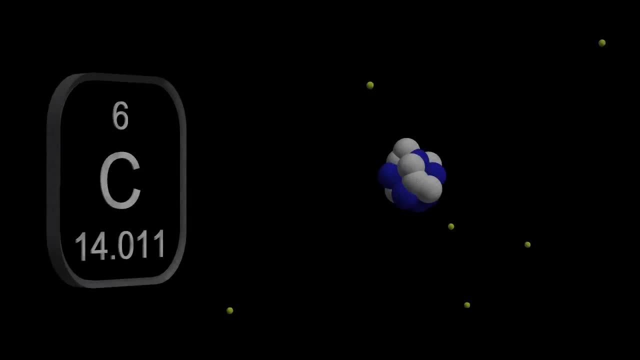 through beta minus decay with a half-life of 5730 years. For the remaining nuclear decay processes we will again use our carbon-14 atom, but understand that this is for demonstration purposes only. Carbon-14 does not decay by any other means except beta minus, as described above. 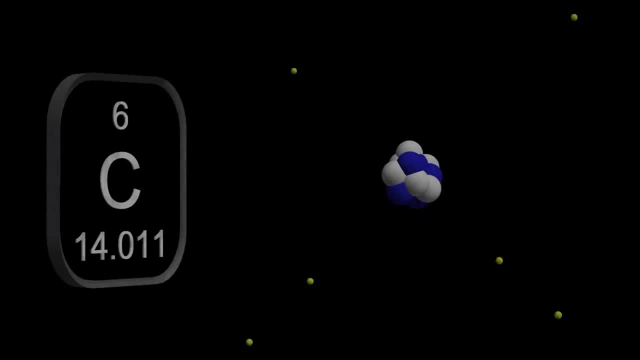 Let's say our nucleus has too many protons and neutrons. These unstable atoms can give off a set of two protons and two neutrons, which is the same as a helium nucleus, This bulky particle with four subatomic units, including two positively charged protons. 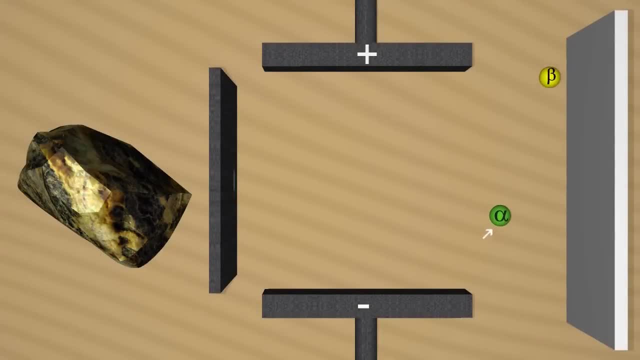 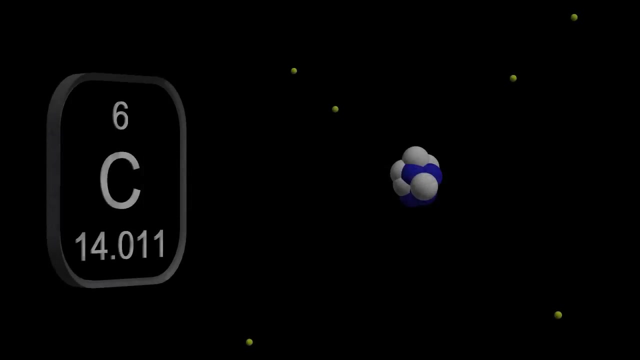 would move relatively slowly and show deflection towards the negative pole of our electric field, corresponding to the alpha radiation described by Rutherford in 1899. Therefore this is referred to as alpha decay. This decay reduces our atomic number by two and reduces our atomic mass by four. 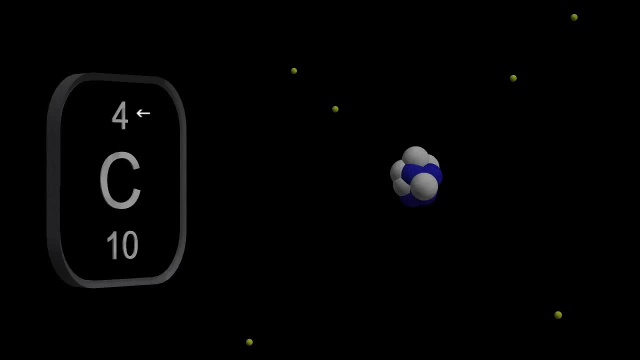 In our example, remembering that the atomic number determines the chemical behavior, our atom becomes beryllium-10,, a known isotope of the stable element beryllium-9,, with a half-life of 1.39 million years. 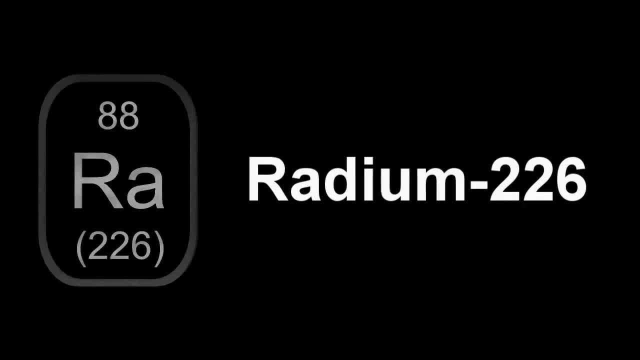 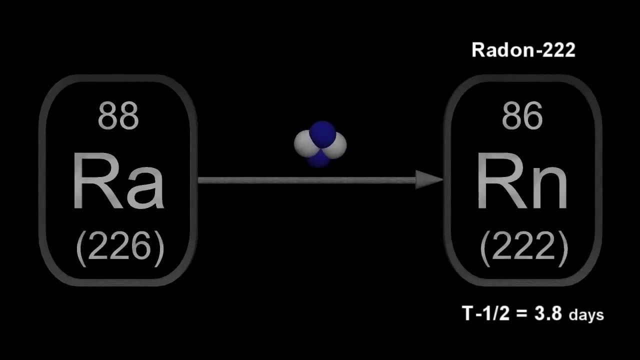 An example of actual alpha decay is radium-226,, which was isolated by the Curies in 1898.. After giving up its helium nucleus of two protons and two neutrons, the new element is the radioactive gas radon-222, with a half-life of 3.8 days. 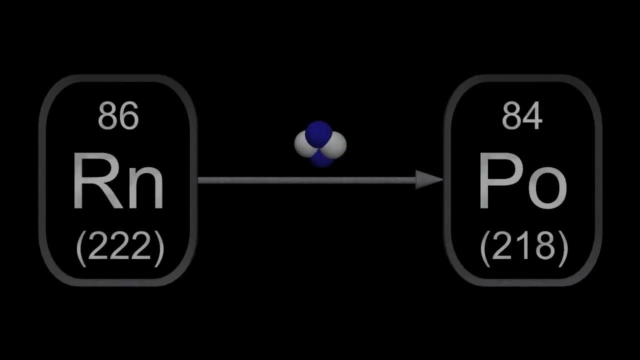 This too undergoes alpha decay to produce polonium-218,, an isotope of polonium-210,, the other element discovered by the Curies in mid-1898.. As these elements transmute, there is matter and energy shifting around inside the nucleus. 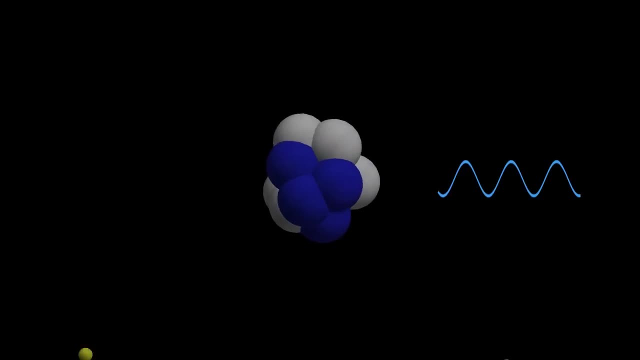 with neutrons turning into protons and vice-versa. Occasionally, there is some excess energy left over after these transformations that the atom needs to expel. This energy is dissipated in the form of an electromagnetic wave with penetrating properties similar to X-rays. 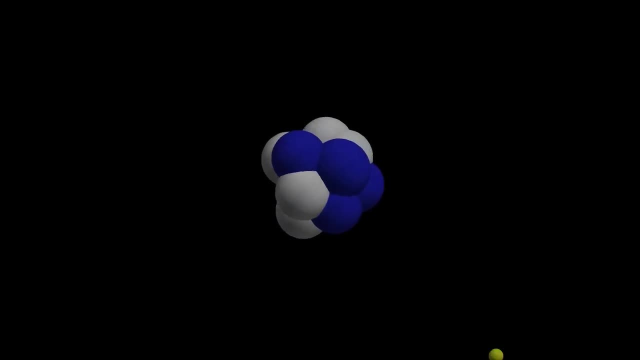 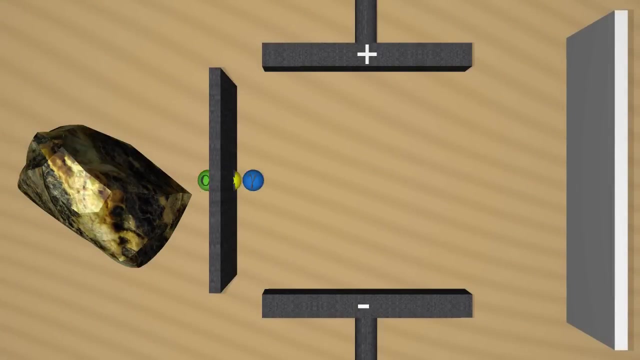 The waves are electrically neutral and therefore are not deflected in an electric field. These waves correspond to the gamma radiation discovered by Villard in 1900 and named by Rutherford in 1903. Therefore, this type of decay process is named gamma decay. 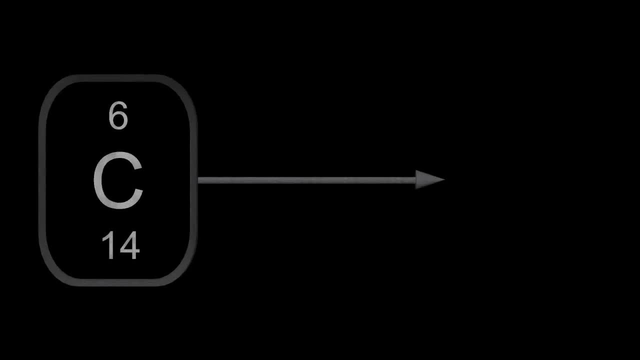 Since the contents of the atom itself are unaltered, the atomic number and the atomic mass remain the same. We usually denote the parent atom with a small letter m after the atomic mass, which stands for metastable, indicating the excess energy content of the nucleus. 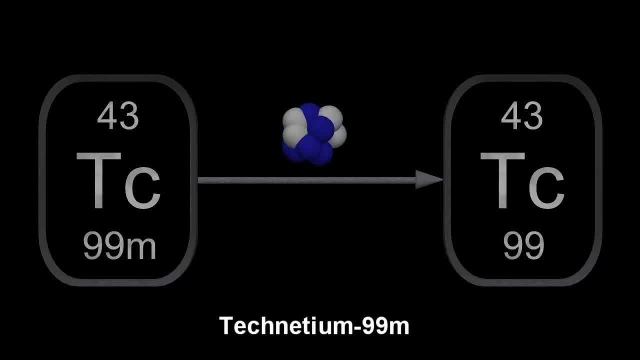 The most familiar element in this category is technetium, the workhorse of medical nuclear imaging. With a half-life of 6 hours and essentially pure gamma radiation production, this particular element is well suited to evaluate various physiologic processes in the body. 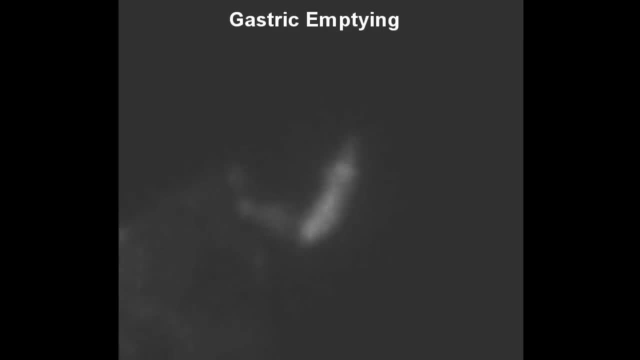 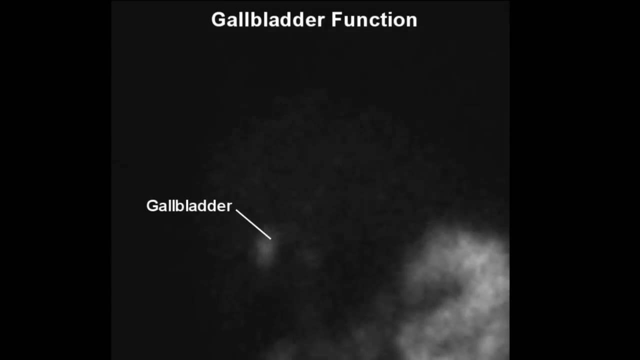 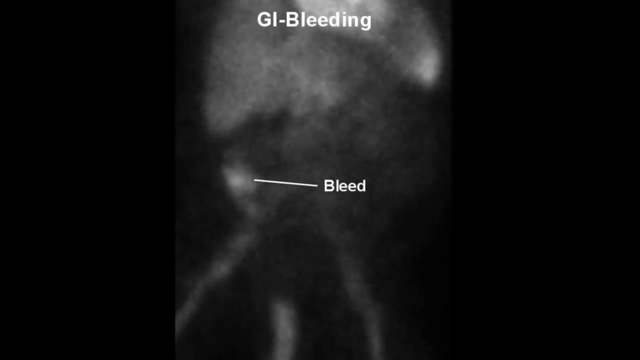 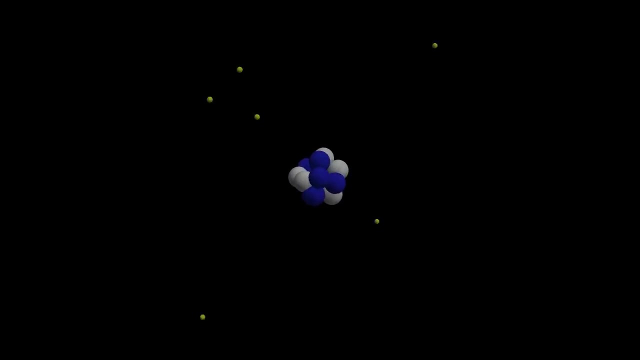 such as gastric emptying, gallbladder function and gastrointestinal bleeding. The last decay processes deal with unstable isotopes with too many protons in the nucleus. There are actually two types of decay that facilitate this transformation, depending on the energy differential between the parent and daughter nuclei. 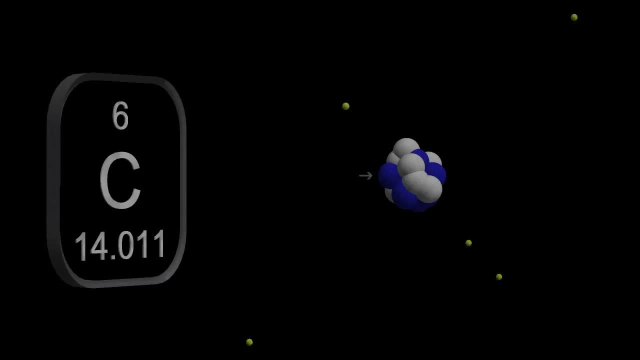 If there is sufficient energy available. one of the protons is converted to a neutron by giving off a small positively charged particle with a mass identical to the electron, but with the opposite charge. This is called a positron and actually represents the antimatter equivalent. 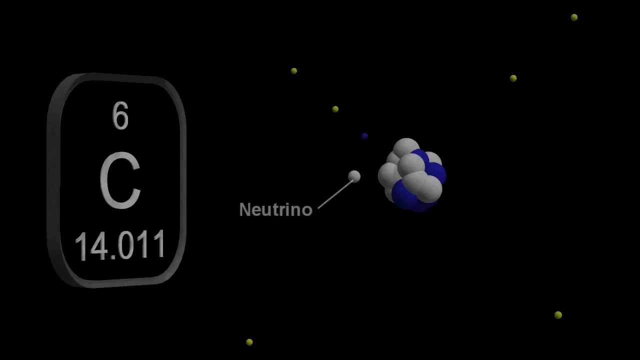 of the electron, The proton also gives up a neutrino, the antimatter equivalent of the antineutrino, to account for the apparent loss of momentum and energy, as seen in beta-minus decay. This antimatter, positron, leaves the nucleus but doesn't travel far enough. 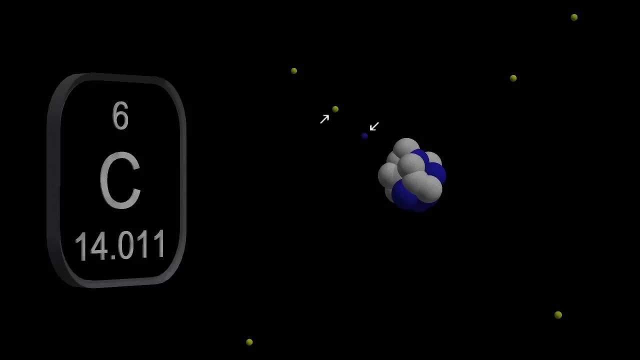 before it encounters one of its negatively charged cousins. in the electron cloud encircling the nucleus itself, The particle and the antiparticle collide, annihilate one another and convert all their mass into pure energy, producing two identical 511 kiloelectron-volt X-rays. 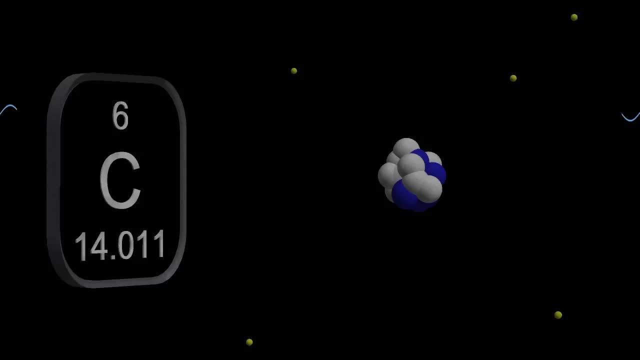 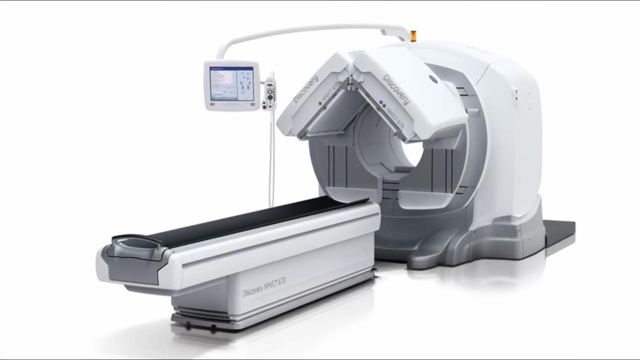 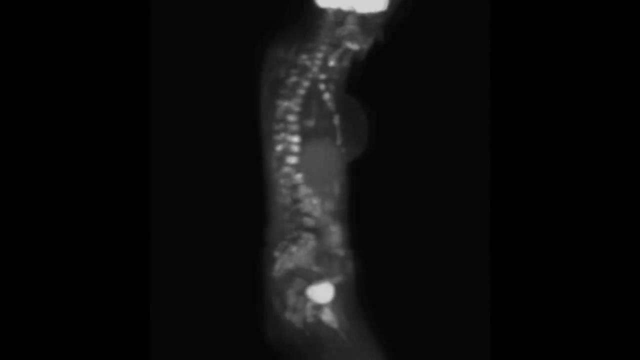 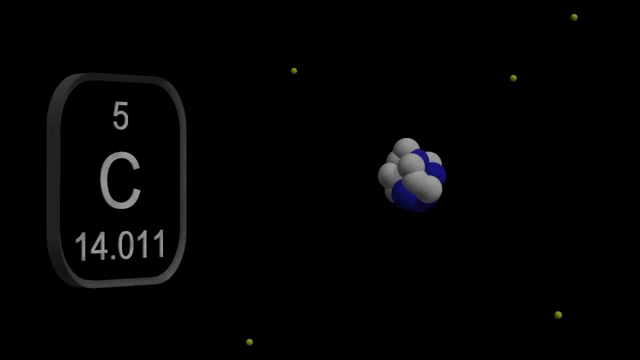 which propagate away from one another 180 degrees apart. These rays can be picked up by a specialized PET or positron emission tomography camera to produce PET images of the body. This conversion drops the atomic number by one but keeps the atomic mass essentially unchanged. 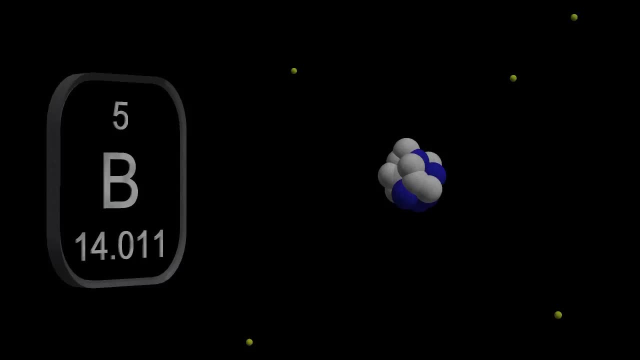 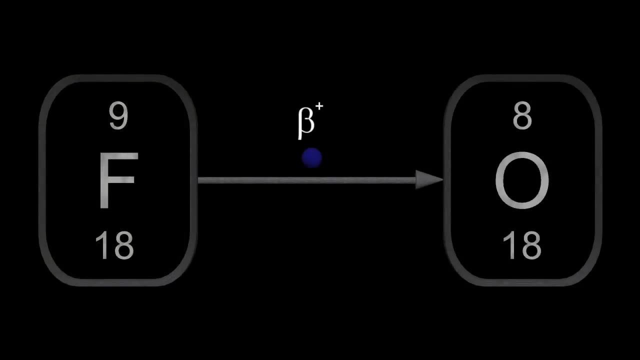 An example of this type of decay is the fluorine isotope F18, which transmutes to the oxygen isotope O18 through beta-plus decay and is one of the common elements used in PET imaging via the agent FDJ or fluor-deoxy-glucose. 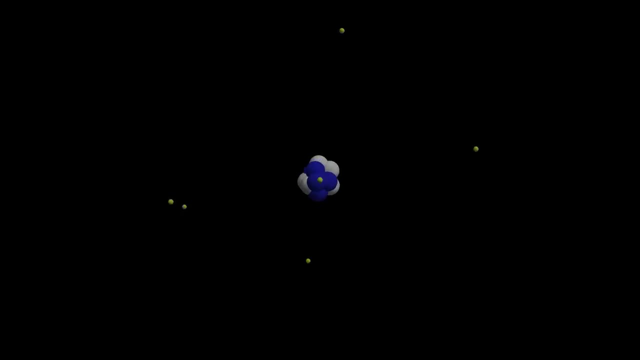 For those paying attention, you may notice that this particular transformation appears to create mass out of thin air. Remember that the neutron, of course, has an atomic mass number of 100% of the neutron, The proton, 99.86% of the neutron. 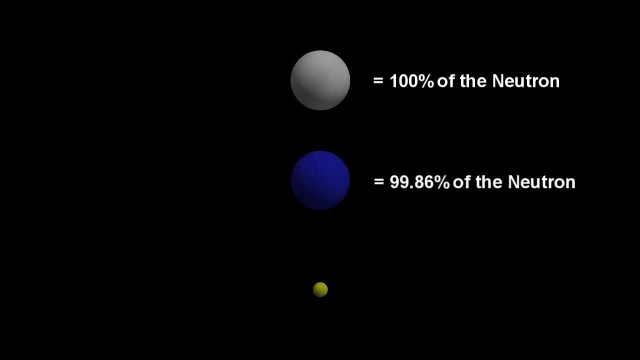 and the electron and positron, 0.054% of the neutron. From a mass standpoint, converting the proton to a neutron and giving off a positron and a neutrino doesn't seem possible. However, as the nucleus becomes more stable, 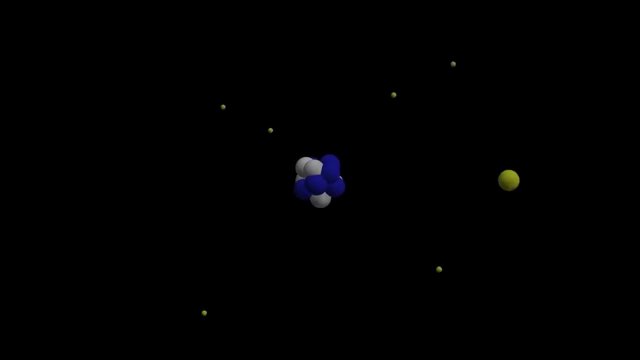 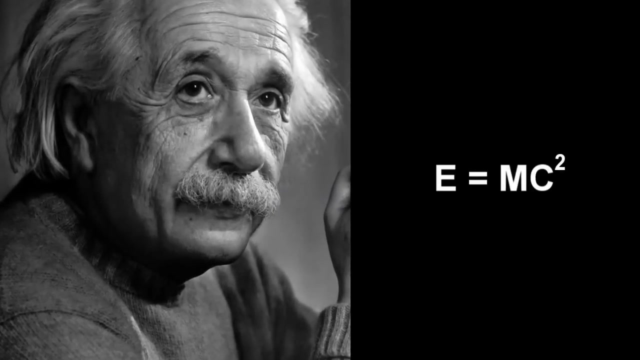 some of the binding energy of the protons and neutrons is converted to mass. according to Einstein's equation, E equals mc squared and can make up for this, Not to get into too much confusing detail, but I do think. a brief discussion of elemental atomic particles. 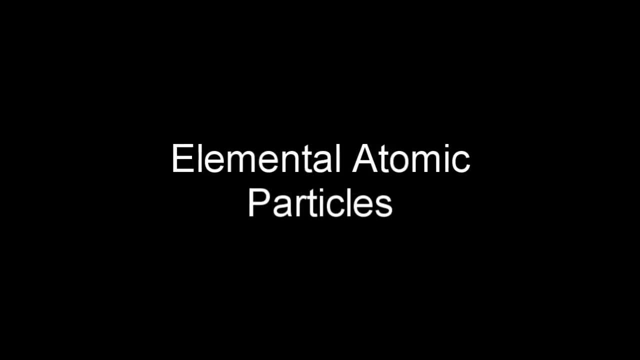 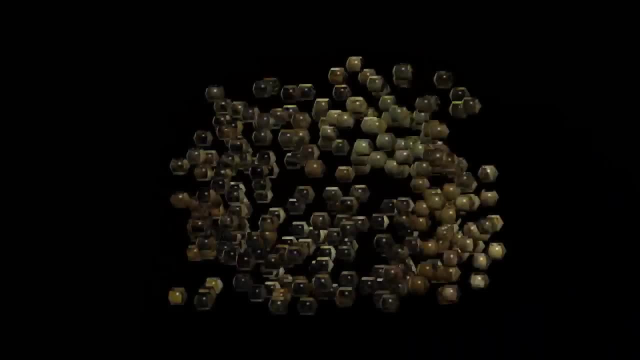 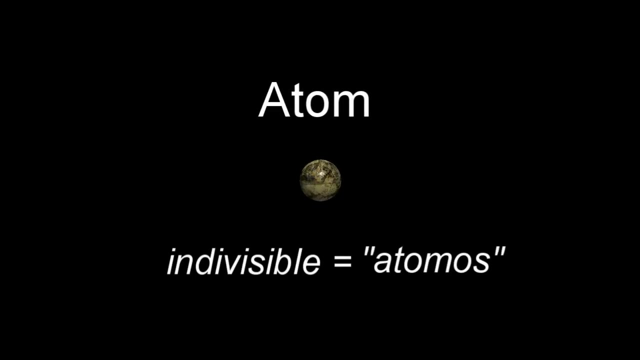 is warranted to explain the phenomenon. The ancient Greeks called the smallest indivisible element of matter, such as this rock fragment, an atom. In fact, the Greek word for indivisible was atomos. Since Rutherford, we now know that atoms are made up of smaller elements. 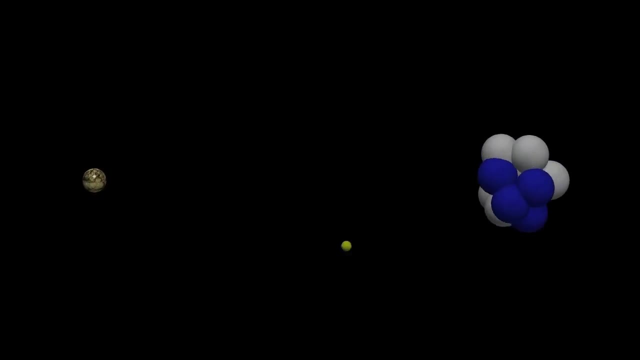 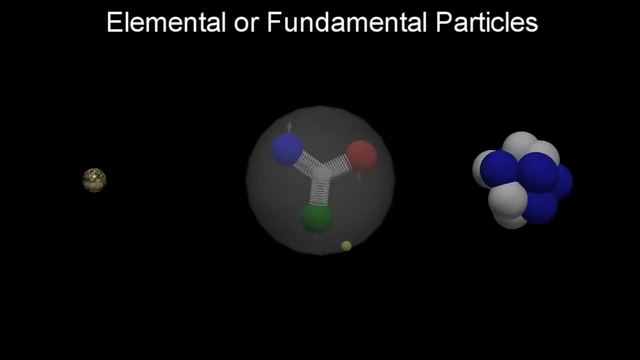 called subatomic particles and are called atomic particles. But what about atoms? What about subatomic particles, the proton and the neutron? Modern atomic theory states that the proton and neutron are made up of even smaller elemental or fundamental particles, so-called, because they are truly indivisible. 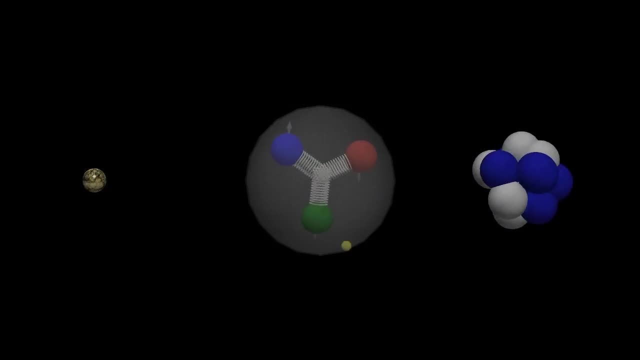 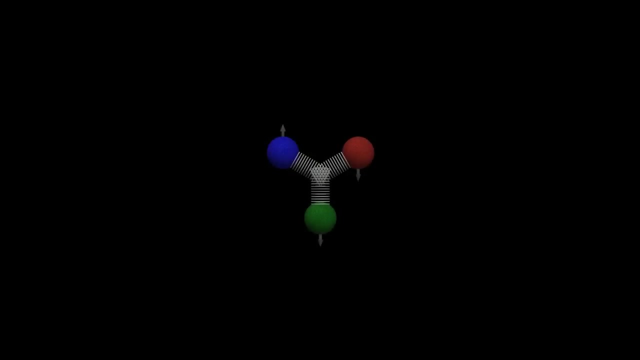 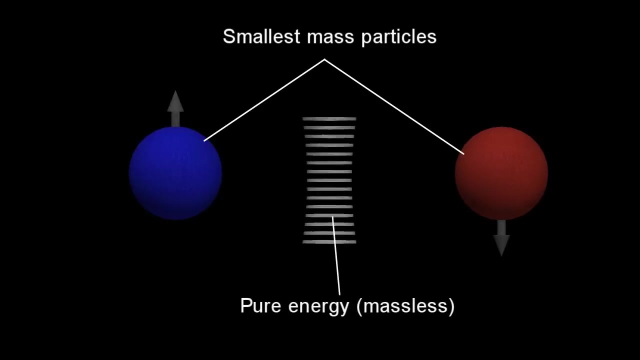 and are the fundamental structures linking energy and matter. These structures include quarks and gluons, as well as the orbiting electron itself. Quarks are the smallest known particles to exhibit measurable mass, whereas the massless gluons are apparently pure energy and 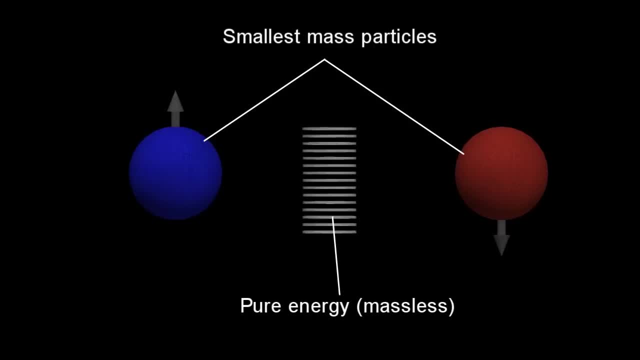 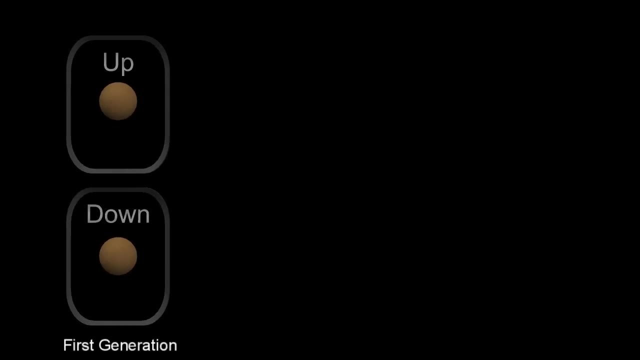 as the name implies, are the forces that hold or glue the fundamental particles together to create protons and neutrons. Quarks come in six types or flavors, including the first generation, up and down, second generation, charm and strange, and third generation. 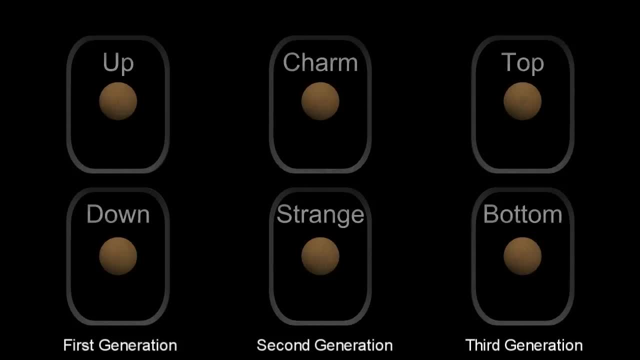 top and bottom. The upper quarks all have an unusual charge of plus two-thirds and the lower quarks all have the equally unusual charge of minus one-third. The absolute mass of the particles in mega-electron volts is shown below each particle. 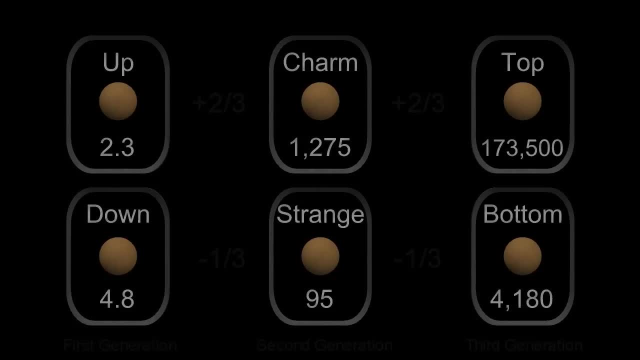 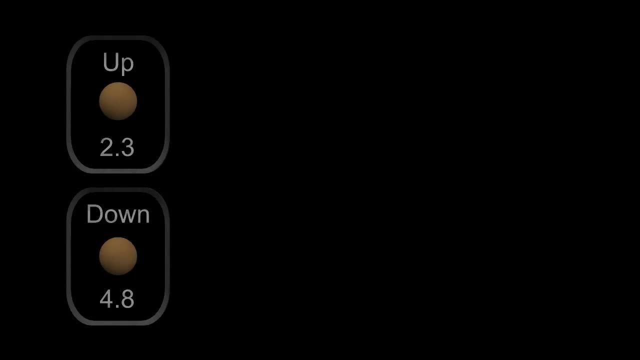 In nature. the only two quarks that are found in abundance and are the basic building blocks of the neutron and proton are the up and down flavors, so we'll ignore the other types for now. We will represent the up and down quarks graphically, with arrows, as shown. 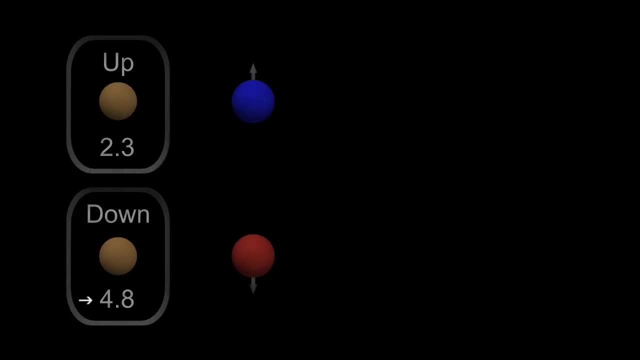 Note that the down quark has more than twice the mass of the up quark, which will be important when we talk about the relative masses of the proton and neutron in a moment. Each subatomic particle is made up of three quarks, held together by three gluons. 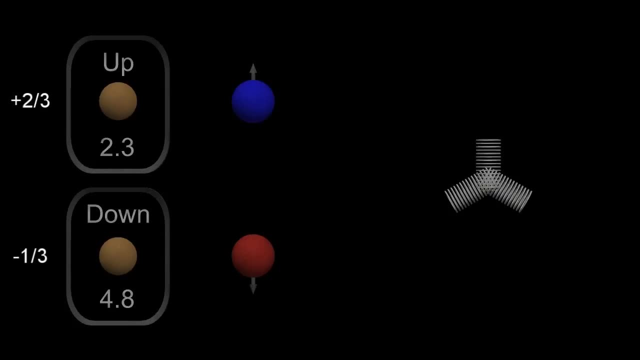 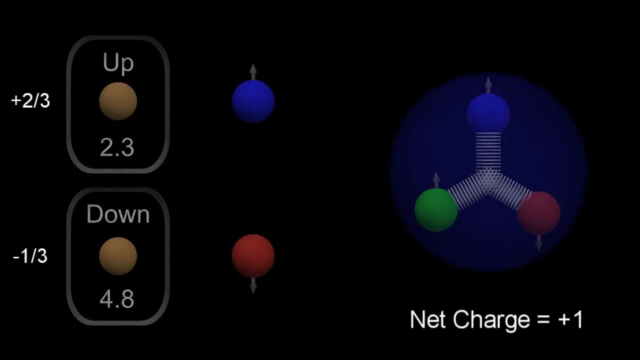 In a proton there are two up quarks and one down quark. Here are the results of the classical authority of Newton. The neutron is made up of one up quark and two down quarks, Adding up the charges of the fundamental particles. 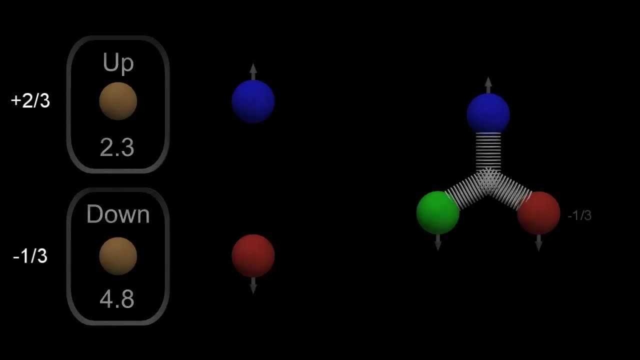 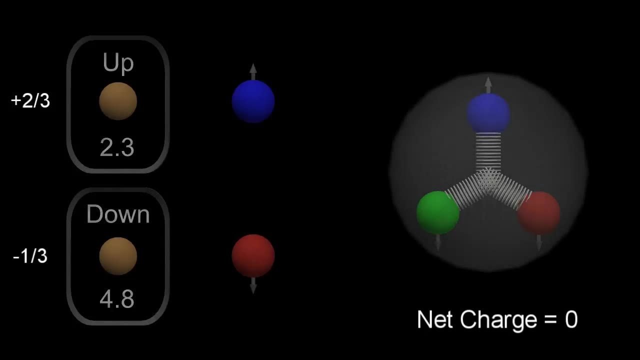 this configuration provides a net charge of plus one: fundamental particles. this configuration provides a net charge of zero, hence the neutral neutron. Remember also that the addition of a down quark provides extra mass to the neutron and at least partially accounts for the mass differential between the proton and neutron. 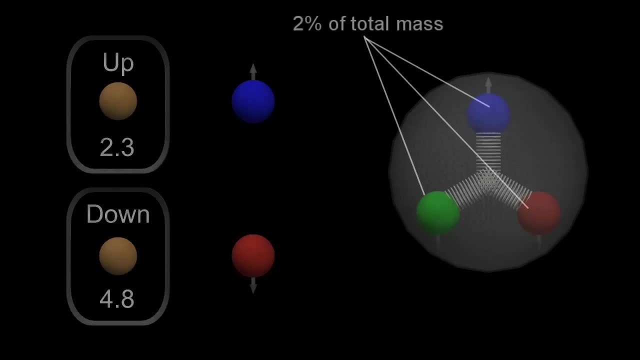 Interestingly, however, the quarks only make up about 2% of the total measured mass of the protons and neutrons. The remaining 98% appear to arise from the pure energy massless gluons holding the quarks together. The gluons, therefore, may be the link between energy and matter, as predicted in Einstein's. 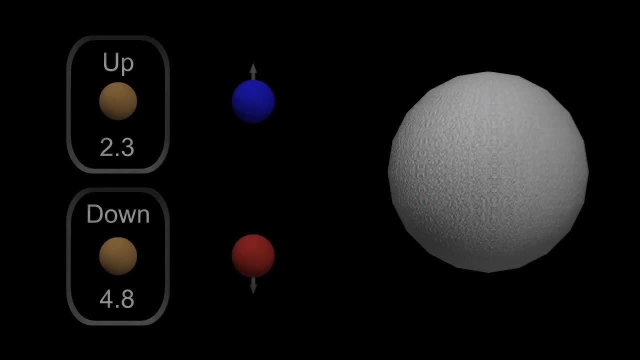 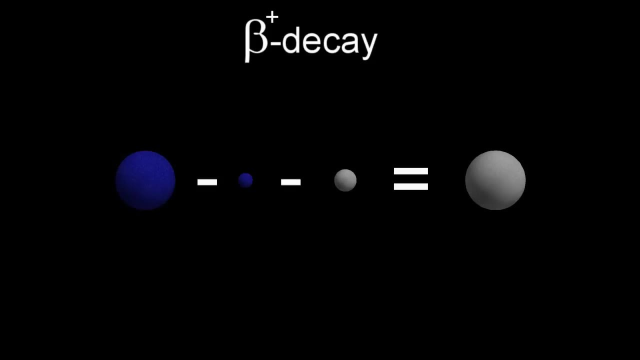 famous equation. In summary, the apparent mass deficit and beta positive decay shouldn't bother you, as the process likely involves some mass generation from the excess energy produced as the nucleus decays to a more stable state For isotopes with excessive protons but insufficient energy to undergo beta positive decay or 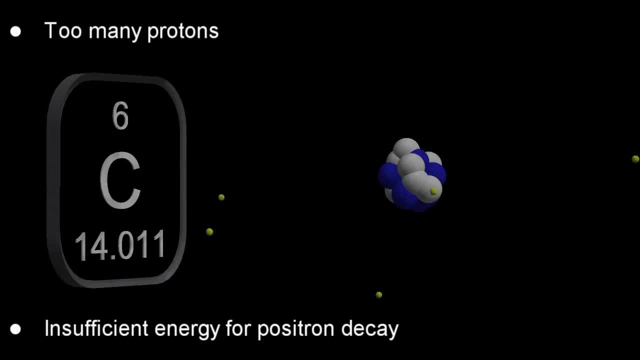 positron emission. an alternative mechanism is available, called electron capture. In this decay process, the nucleus captures an inner shell orbiting electron which is absorbed by the excess proton. The proton is converted to a neutron and the nucleus emits a neutrino. In addition, one of the outer shell orbiting electrons is absorbed by the outer shell of. 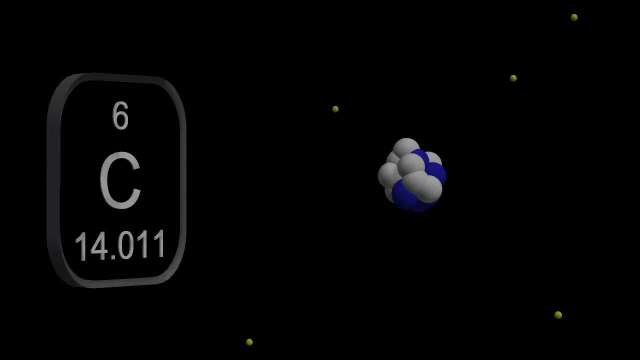 the neutron then falls into the vacant inner shell and gives up energy in the form of an electromagnetic wave. Remember that the only difference between an X-ray and gamma ray is where they are produced. Gamma rays are produced in the nucleus of the atom, as it gives off excess energy. X-rays 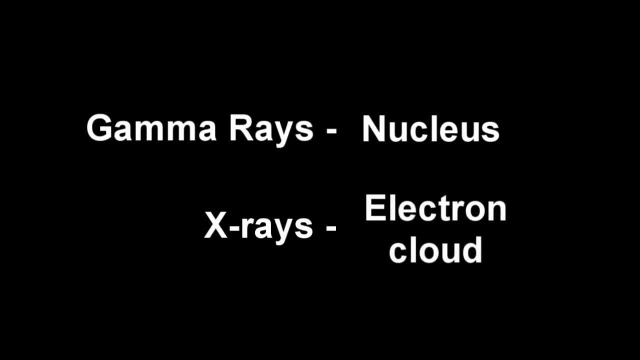 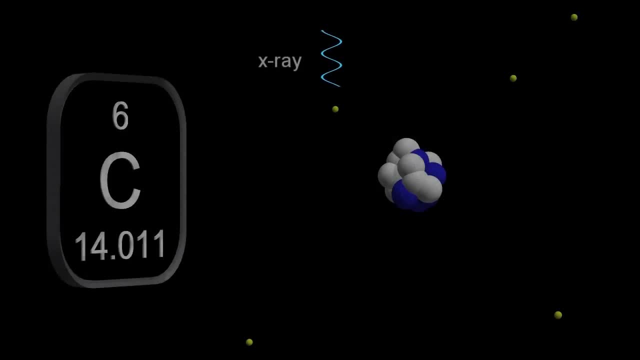 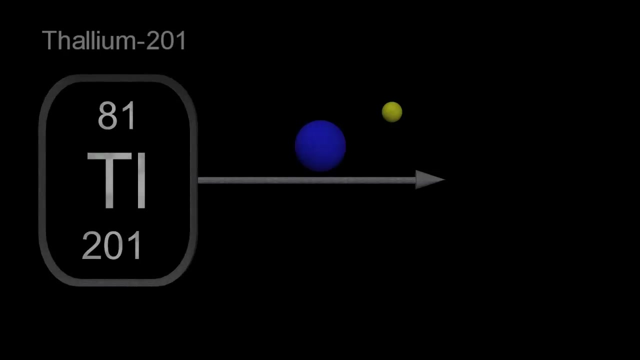 on the other hand, are produced in the electron cloud. Therefore, electron capture actually produces X-rays. as the outer shell, electron falls into the inner orbit Under depositron emission. the atomic number decreases by one, but the atomic mass remains unchanged. A clinical example is thallium-201,, which decays to mercury-201 and produces mercury.